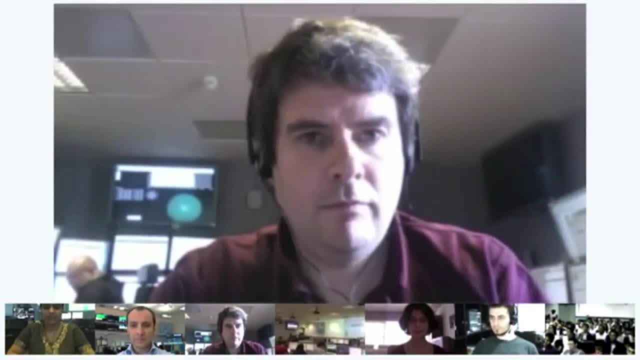 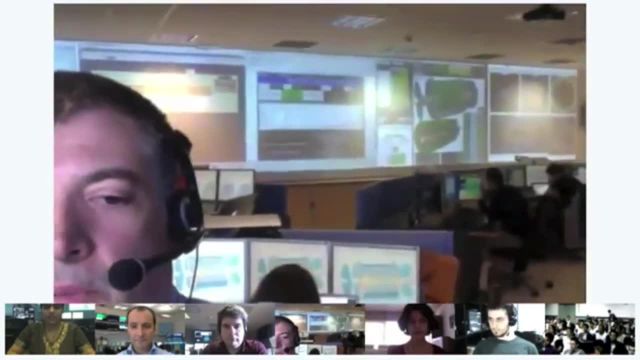 And so you can take a look at our control room here. Just give you a quick glance, And we're just here, ready to go, waiting for those stable beams that we've been promised, and we're ready to start the data. Oh gosh, you're right, It's my fault. 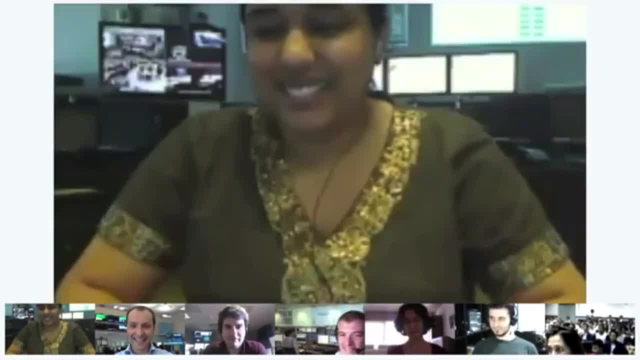 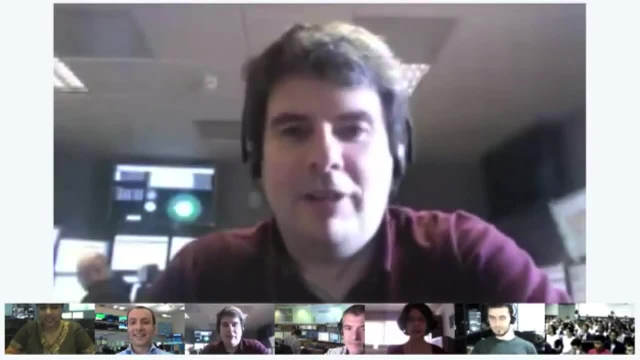 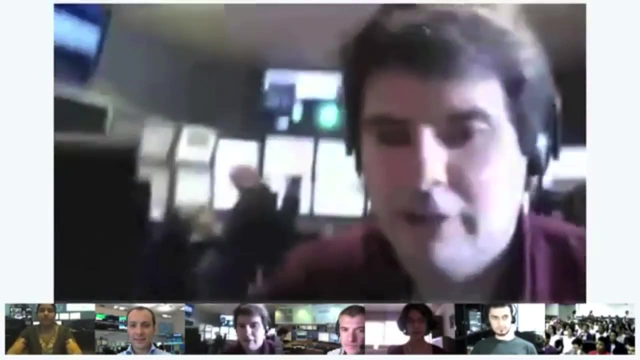 Soon after the hangout: right Hi. so now going over to the CMS control room. David, Yeah, so I'm Dave Barney, I'm a physicist for the CMS experiment and I'm here in our control room. I can also show you some of the people on呀. 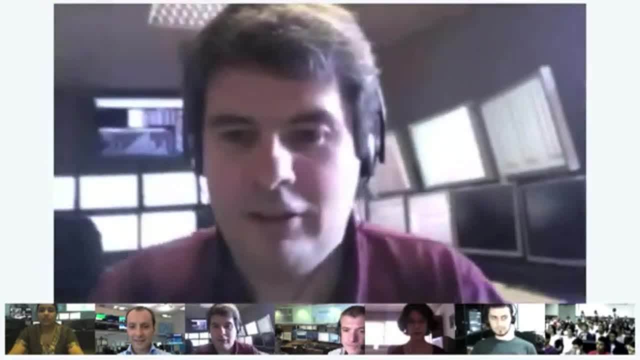 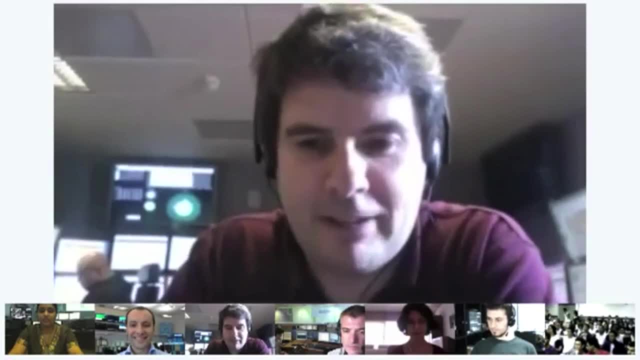 shift behind me. We're also eagerly awaiting these first physicsCH 상. awaiting these first physics collisions of 2012 that Mirko has promised us, But he's gone back on his promise again. We're just waiting for him. Keep waiting, David. 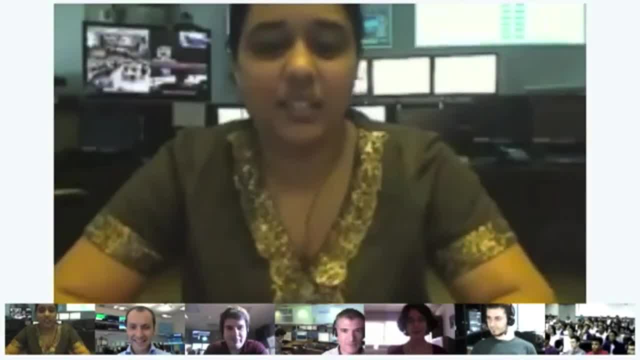 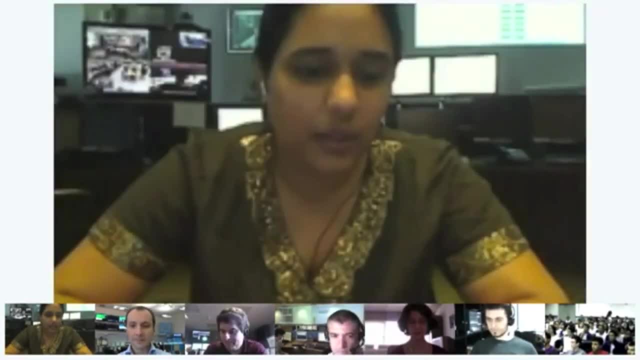 OK, so while we're waiting for the beam, let's see if we can actually have some discussion. I see that our Brazilian friends have already logged in. Can everybody there hear me? Can everybody wave your hands to confirm that you can hear me? 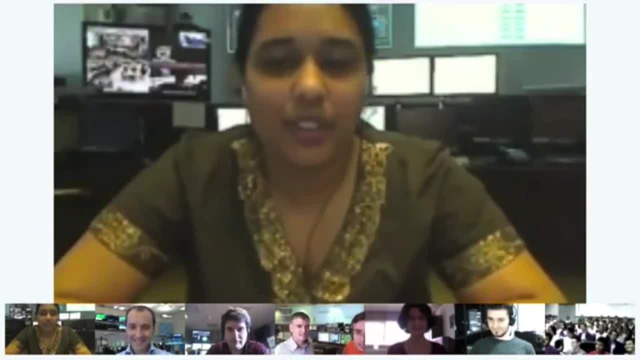 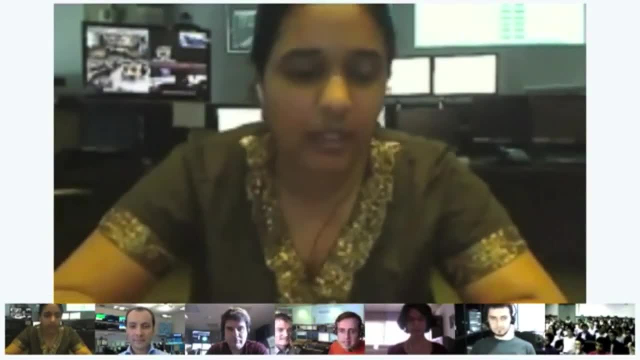 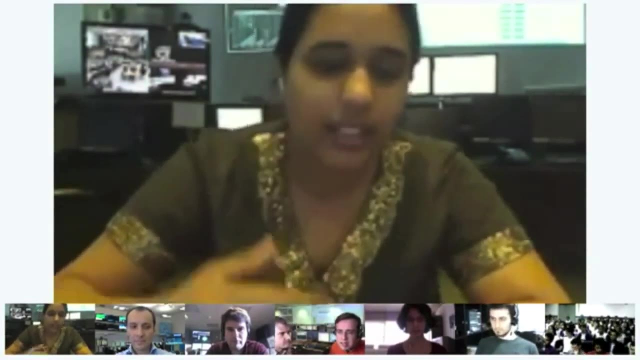 Yay, OK, fantastic, fantastic, OK. so the way this is going to go now is it will be our Brazilian friends first actually asking three questions, and then followed by Lydia asking a question, And then again back to Brazil for a few more questions, and 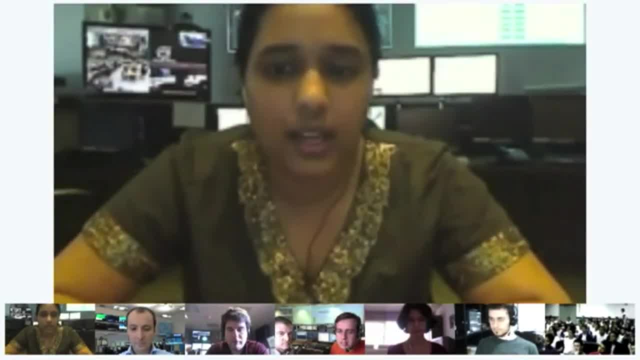 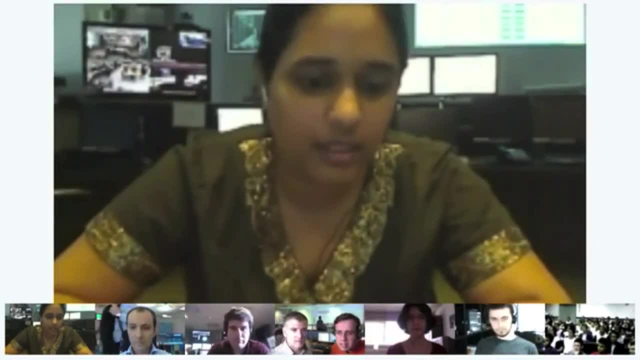 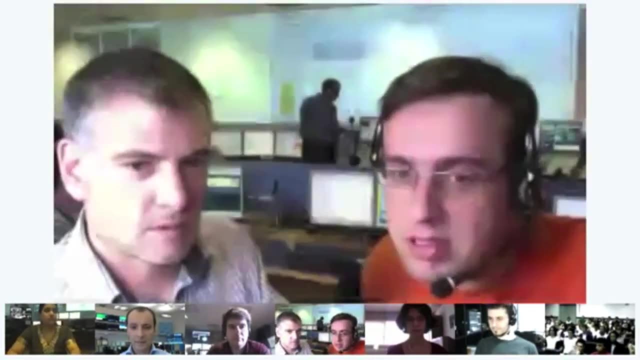 then a few questions. Questions from Don. So let's start with our first question. Can anybody from Brazil actually confirm and say something that they will be asking a question? I hope they're going to ask in English, I don't know, OK. 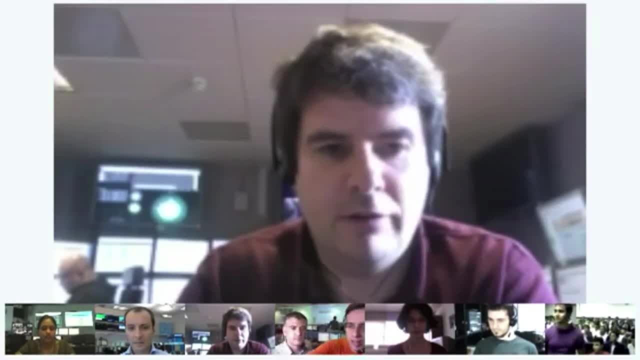 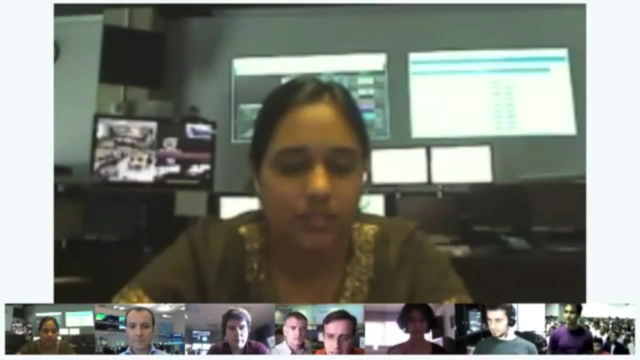 We can just about hear you, but you're very quiet. Yeah, Hello, can you hear me? Yes, Can you come a little bit closer to the mic please? Hello, can you hear me Loud? Yes, A lot better now. 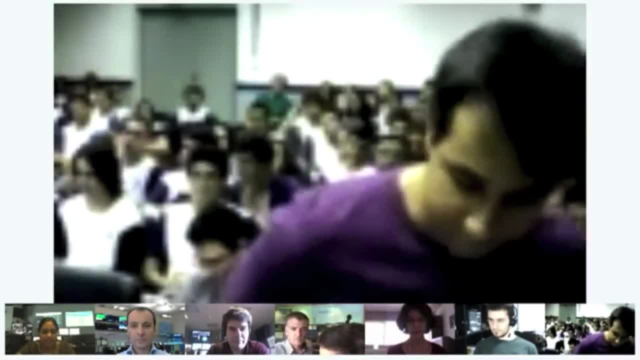 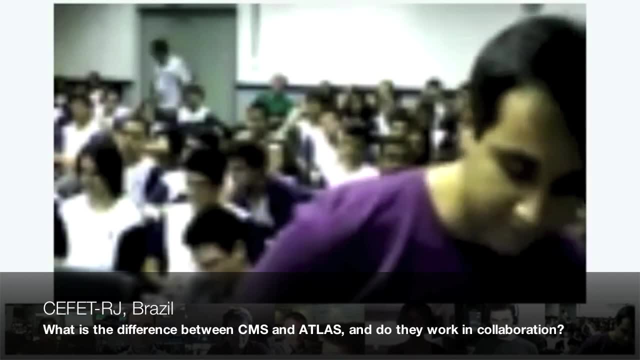 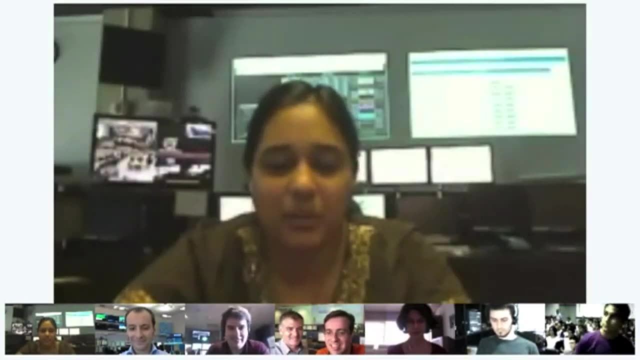 OK, OK, OK, I'm going to make my first question. I want to know what's the main difference between Atlas and CMS, and I want to know if they work in collaboration. OK, I think, to be fair, I will split this question into two. 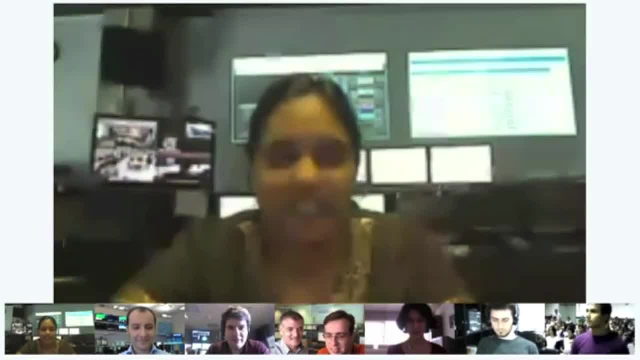 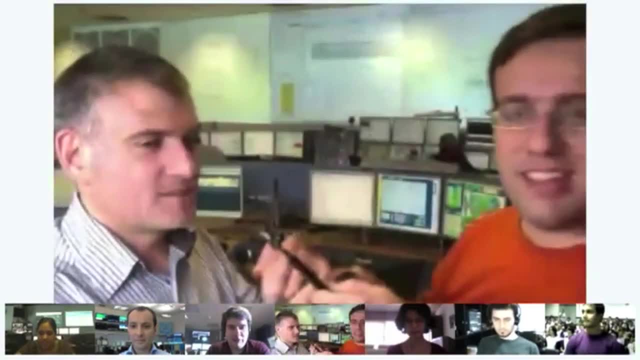 parts One is that we have two experiments, and I think that we can let both David and Steve answer this. So David first. OK, So I could be politically incorrect and just simply say that CMS is so much better than Atlas. but oh, I've said that. 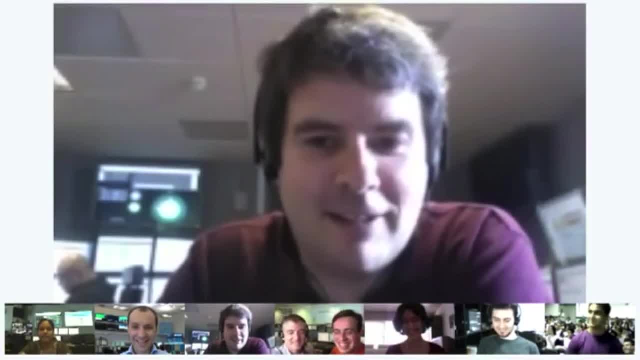 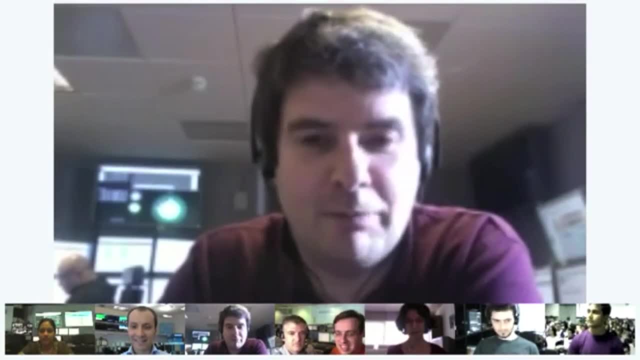 Sorry. So what we do is we have at least two experiments, trying to look for the same things but built in different ways, And the reason for that is we're trying to look for the same things but built in different ways, And the reason for that is we're trying to look for the same things but built in different ways. 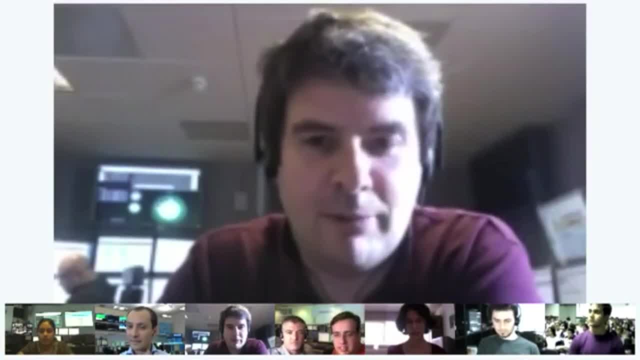 And the reason for that is we're trying to look for the same things but built in different ways. And the reason for that is when you're at school doing an experiment, usually your teacher knows the answer, So you have something to compare your results against. 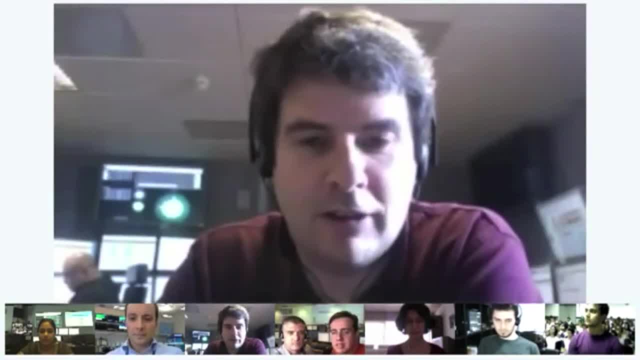 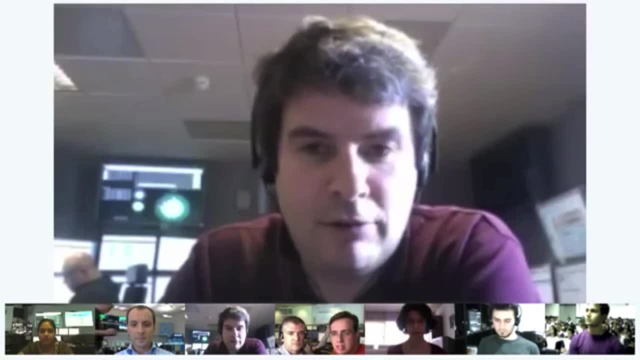 What we do is completely new. We're looking for things that no one has ever seen before, And looking for well, sometimes we don't even know what we're looking for. So having two experiments confirm each other. So if one gets the result and the other one doesn't see the same thing, it's probably 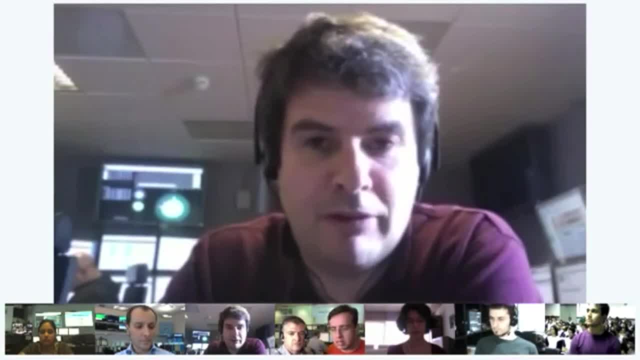 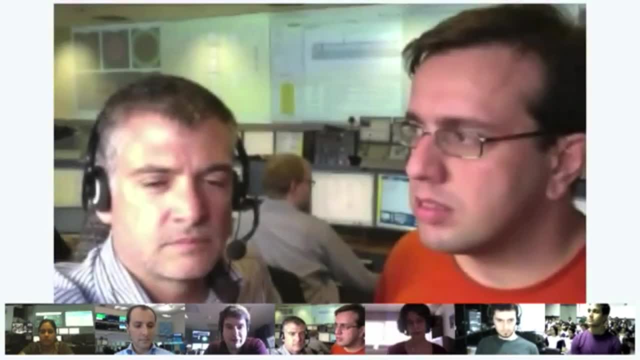 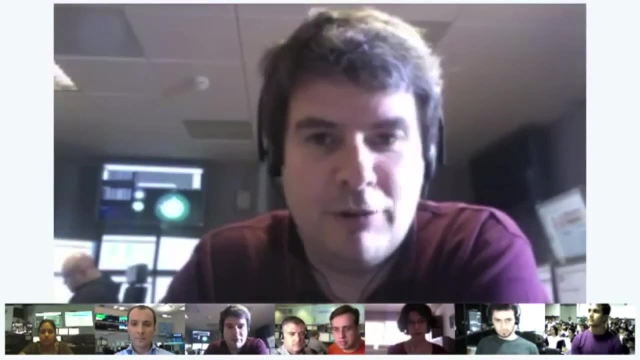 not real, Whereas if both experiments see the same thing, you can pretty much be sure that you've seen something real and maybe new physics. So having two experiments is a great thing to have. Ideally you'd have even more, but two's enough for us. 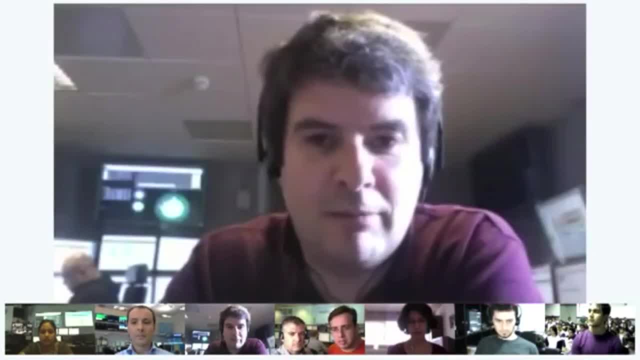 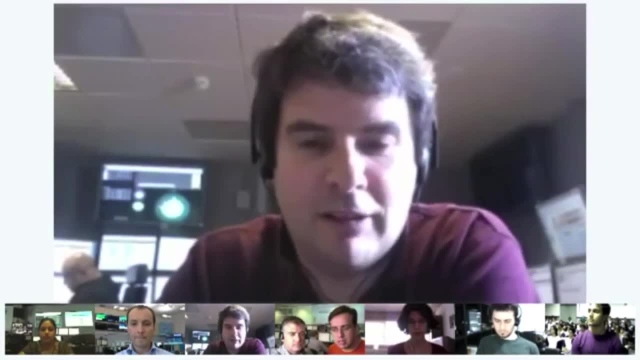 And we build things in different ways. So the aims are the same. The overall structure is very similar for these two detectors, but they're built differently- different Yeah Yeah, Technologies and so on. Maybe Steve can comment a bit more on that. 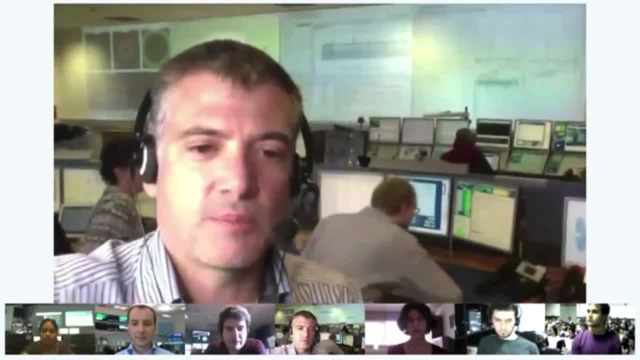 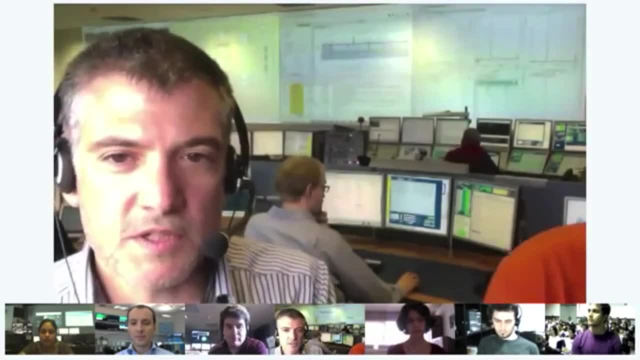 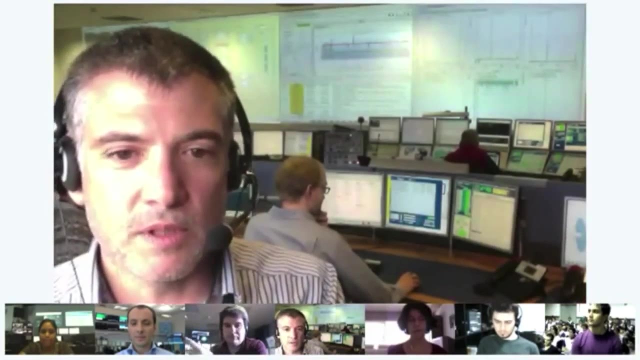 Sure, I would mention that perhaps as important as having different technology is the fact that our 3,000 physicists are completely different than the 3,000 physicists working on CMS, And that's extraordinarily important. We provide checks within our own experiments continually. 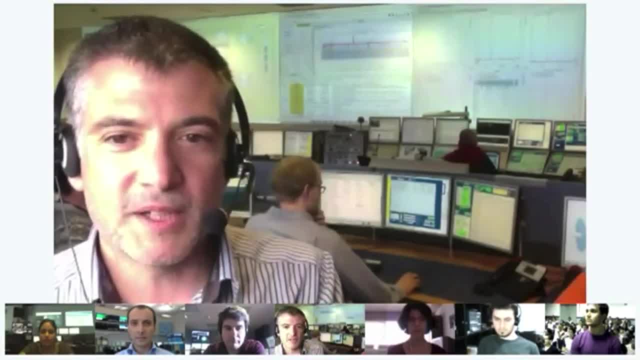 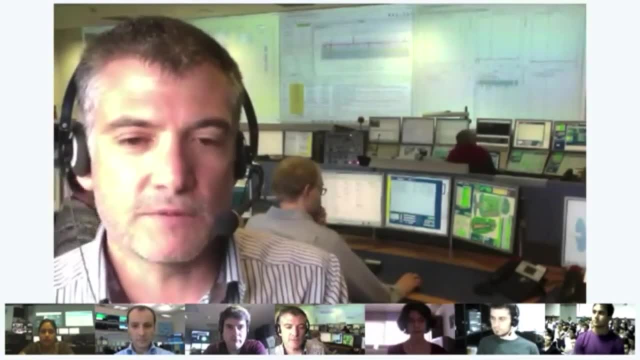 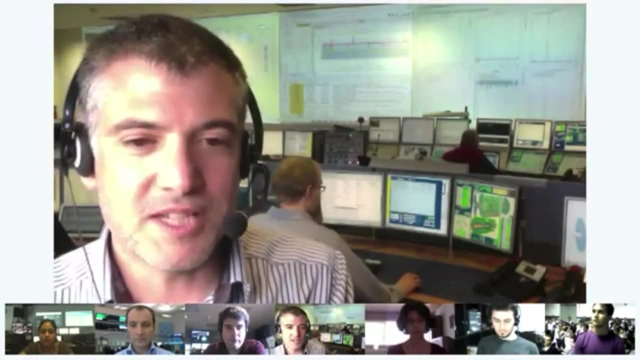 Peer review is probably the most important and powerful tool that we have in science. So we each check our results And, if they survive our own internal reviews, then we compare against each other and we each review and take a look and see if we measure something that's the same or similar. 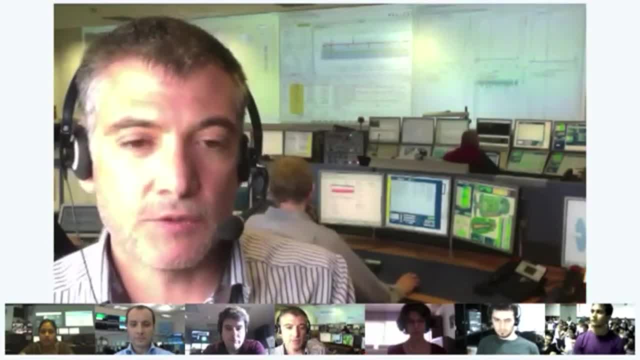 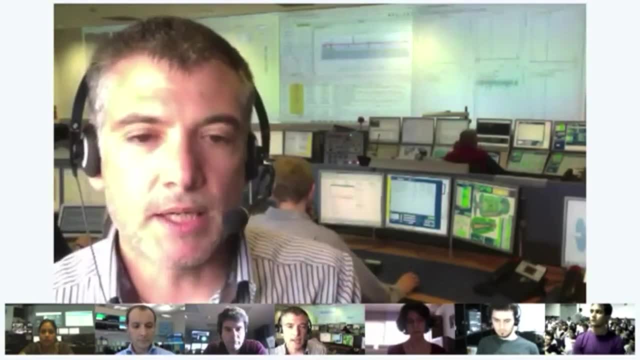 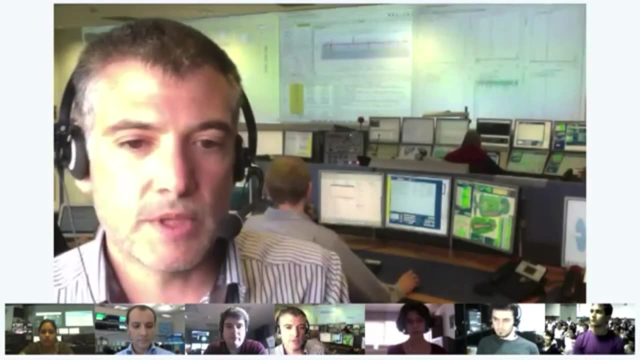 or different. Now, technically, if you look at the two experiments- and I invite you to look at them, take a look on the CMS page, take a look on the ATLAS page- you'll see that they really look different And the driving difference between the two is how they go about measuring the different. particles and detecting them. What drove the different sizes between the two has to do with the magnets. In fact, our acronyms the compact muon solenoid and the ATLAS, which is a toroidal LHC upper apparatus. the name is due to the magnets, the giant magnets which surround the detectors. 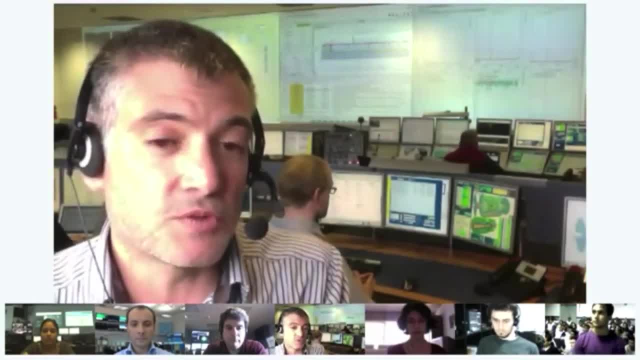 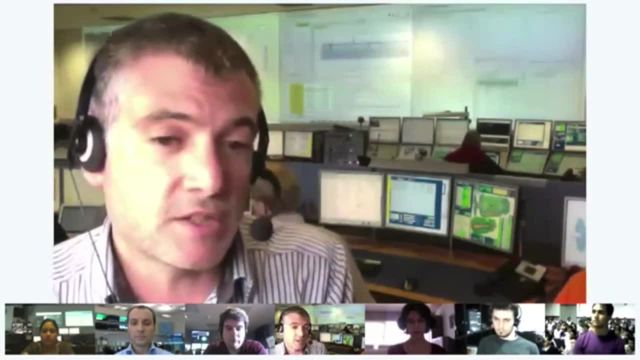 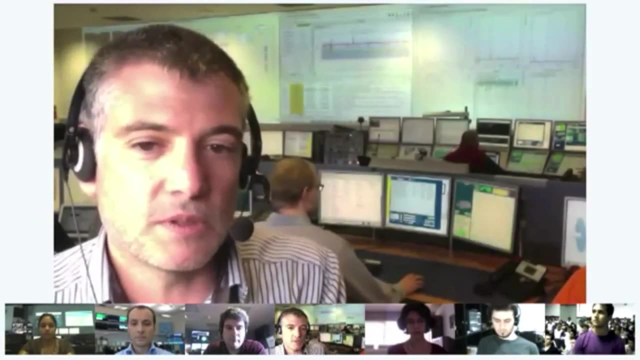 and which curve muons so that we can measure their momentum. That's really the driving force behind the change of the shapes, And that changed the shapes and the types of technologies used inside the detectors. So yeah, the detectors are very different, yet they're both designed to explore. 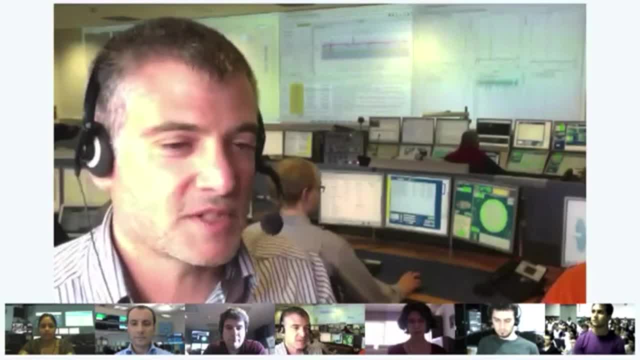 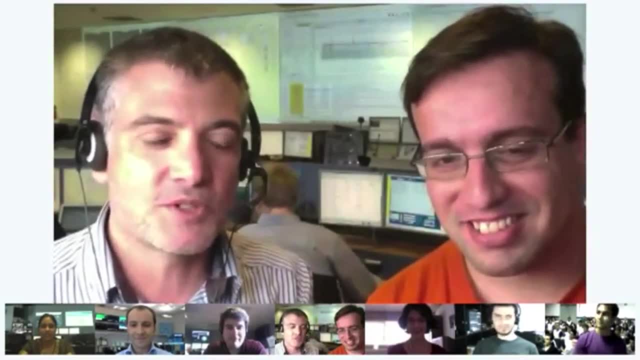 And that's what we're both doing. I wanted to, before stopping, just introduce Dennis, who's here. So if you want to add something to that, Okay. So Dennis asked, in Portuguese also, a question. Dennis helped to make sure that the school in Brazil could join. 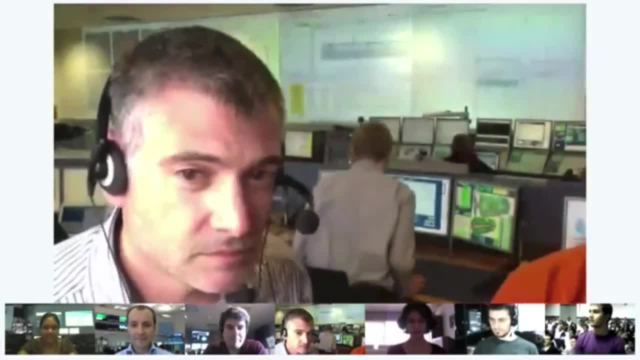 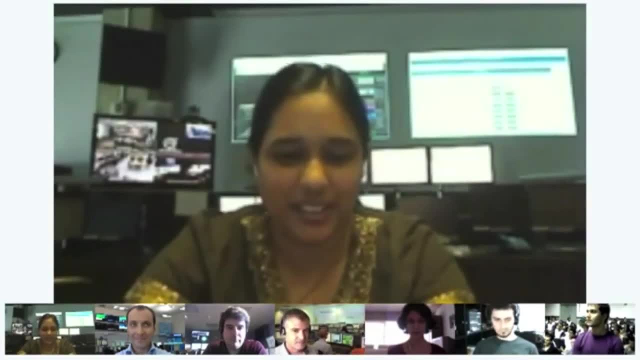 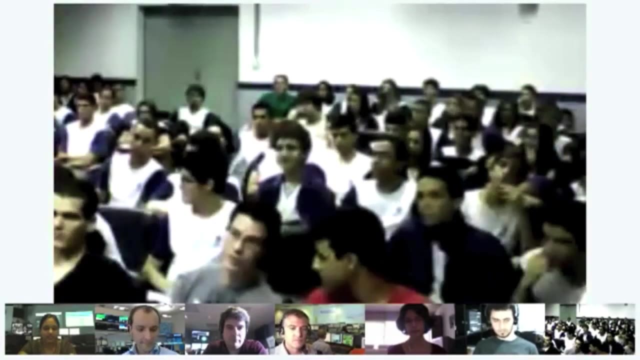 Does that answer your question? Fantastic. So yeah, I guess we all work together in a way that we always cross-check each other. So, going on to the second question, Thank you. Thank you for the answer. So who will be asking the second question? 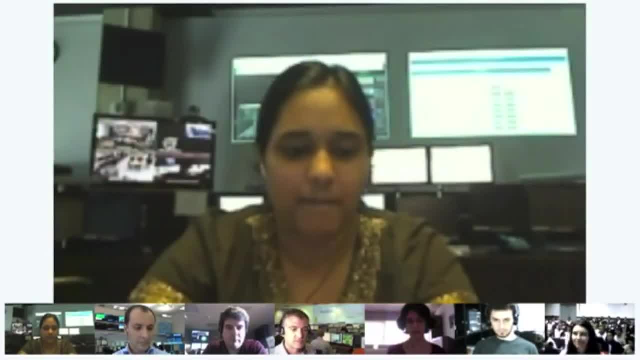 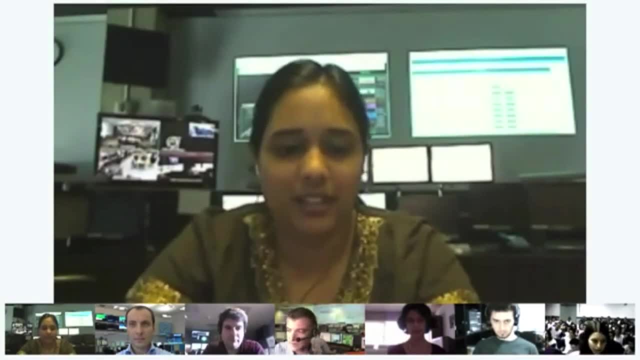 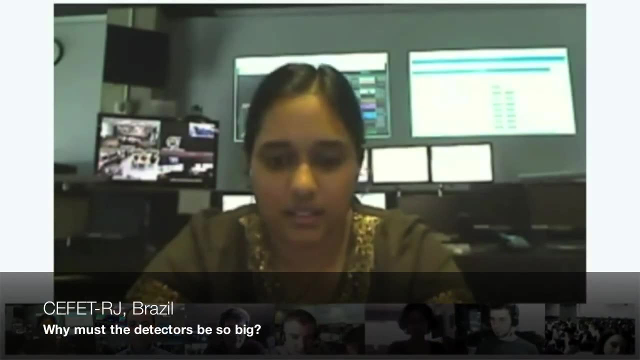 Hi, my name's Laura. Hi, Laura, Can you also please stay a little bit closer to the mike. We can almost hear you. I'd like to ask why the detector must be so big. Okay, why the detector must be so big. 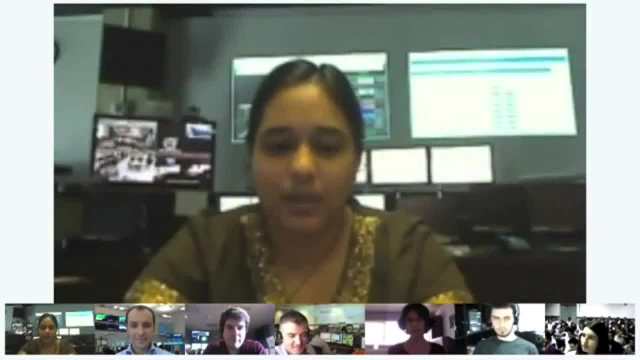 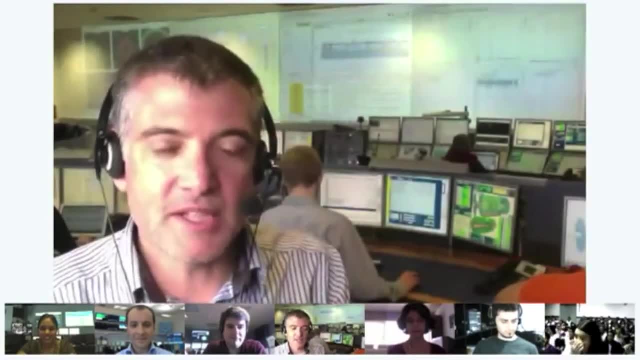 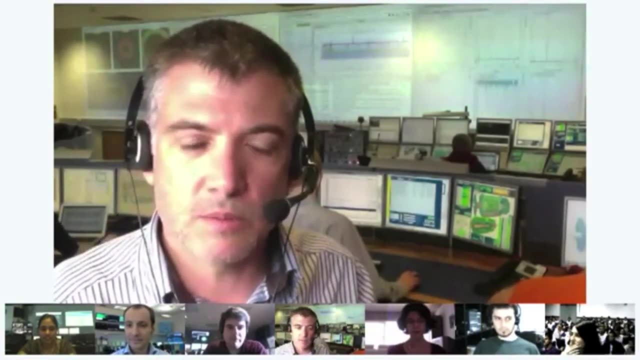 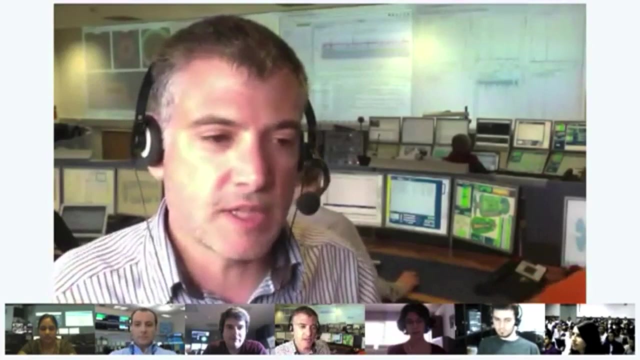 Again, I think this question can be split between Steve and David. Maybe Steve want to go first this time. Okay, Maybe I should. In volume, Atlas has the largest of the experiments In weight. CMS is twice as massive as ours. There's a very good reason for it. As I mentioned, the magnets that surround the detectors have a different shape, and that drives the size. 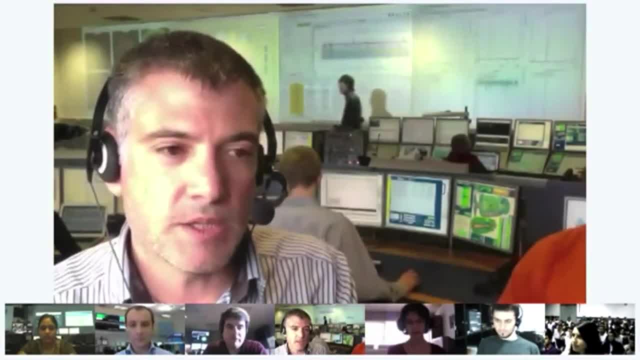 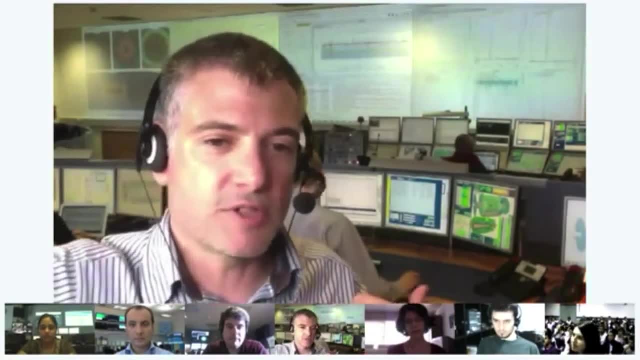 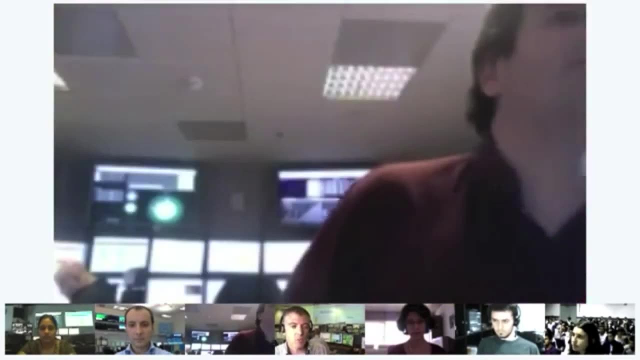 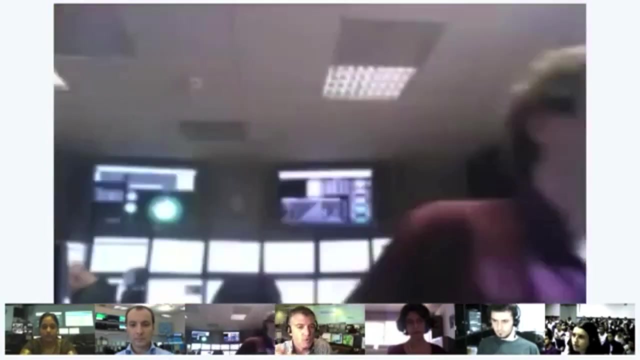 The reason they have to be so big is because we're exploring. It's almost the same reason why telescopes got longer for us to see further out into space. In this case, we're trying to look at particles which are more massive. When a more massive particle, those are the ones we haven't found yet. when a more massive particle decays, the particles that come off of it. when it disappears it shoots off particles and those are going to go very fast. They're going to have a lot of energy. The way we can measure the momentum or the energy of a particle that's charged is by curving it. We do that with strong magnetic fields and the bigger volume you have to measure that curvature, the more precise your measurement is. 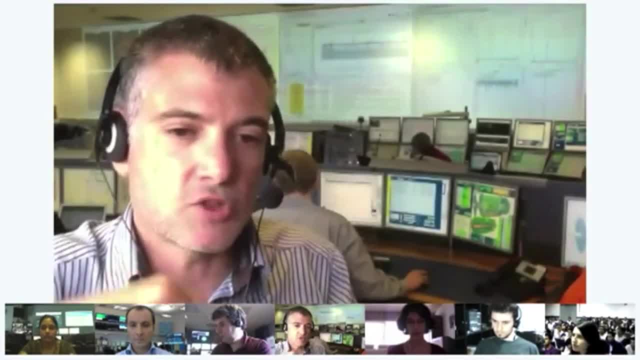 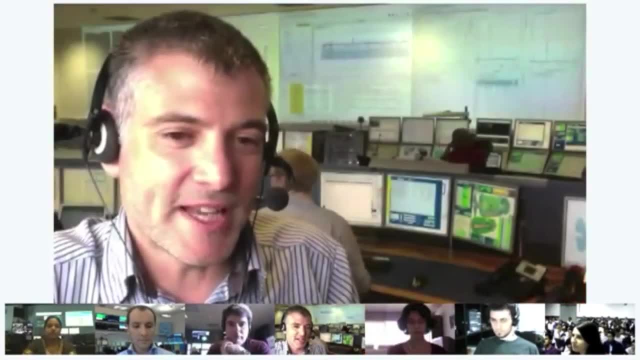 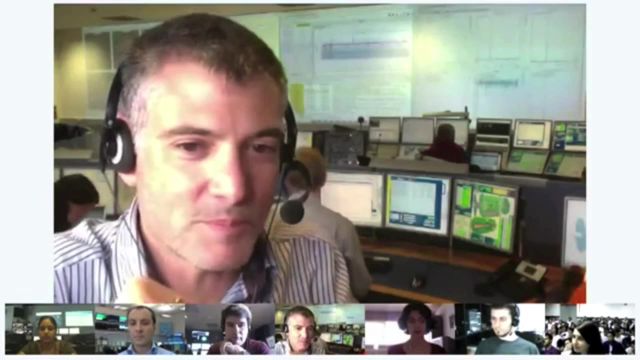 As an example, I think both of our detectors in the tracking parts get down to measuring much more than the actual measurement. If you measure microns of precision- and that's over something for ATLAS- we're 46 meters in length, so if you can measure precisions on the order of microns, over half of a football pitch. 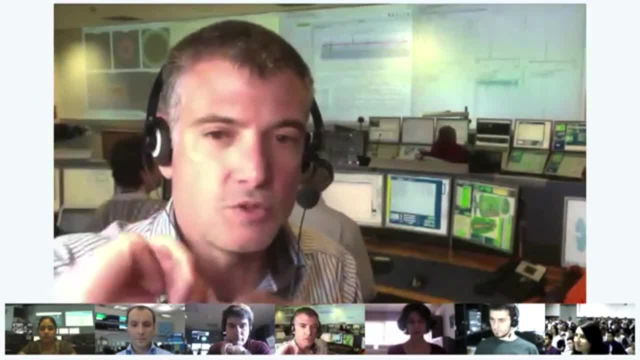 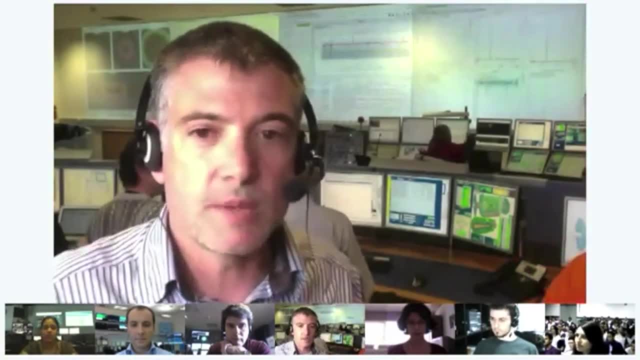 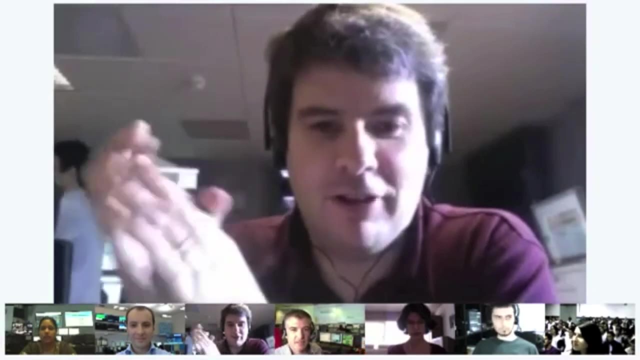 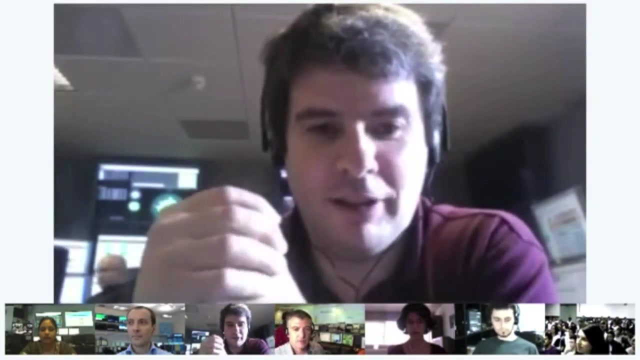 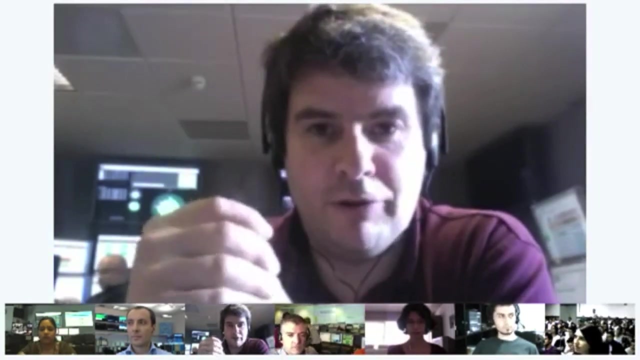 then you can tell one of the new fast-moving particles. you can measure its momentum. So it's necessary to be large to do that. Maybe Dave has a good explanation as well. I think you covered it pretty well, Steve. We don't just build the biggest objects we can make for fun. they're necessarily large. they're necessarily huge because of the huge energies of the collisions that are involved that our friends from LHC are providing us. 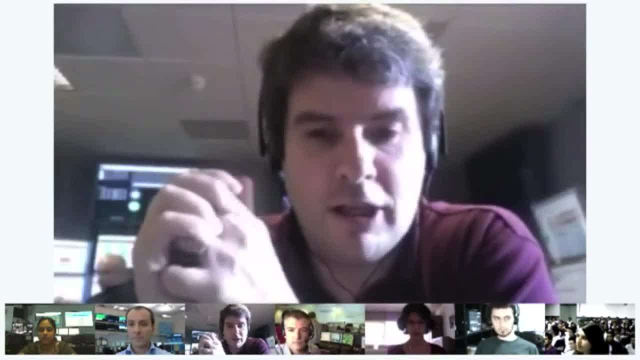 So the particles that fly out are higher energy, higher momentum, traveling faster than anything that's ever been produced in space. So the particles that fly out are higher energy, higher momentum, traveling faster than anything that's ever been produced in space. So the particles that fly out are higher energy, higher momentum, traveling faster than anything that's ever been produced in space. 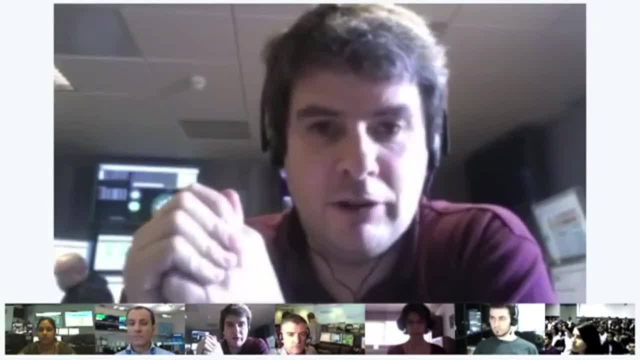 in the lab before. So the experiments that Steve and I work on are the biggest experiments of their type ever made, in fact. So the experiments that Steve and I work on are the biggest experiments of their type ever made, in fact. So their type ever made, in fact. 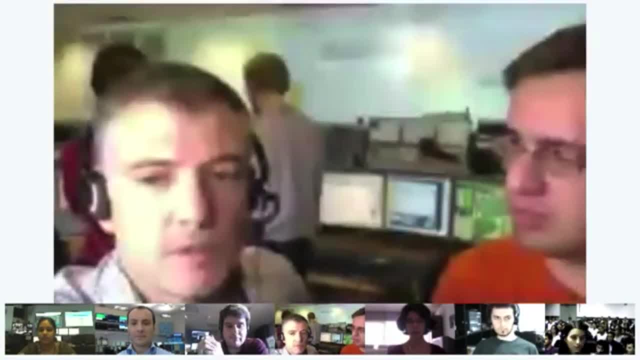 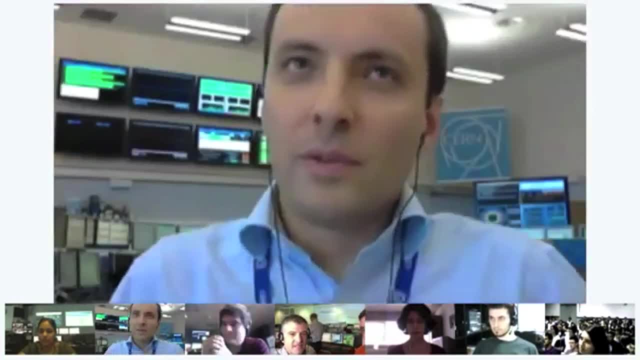 But they have to be like that. Maybe, just maybe Merkle can add why the LHC has to be so big too, just to make it complete. Wow, good question. Okay, if you okay, Let's say like that: If you want to increase the energy of the particles that you are mashing with early on, If you want to increase the energy of the particles that you are mashing with early on one against the other, you have two ways of doing that. Well, essentially, for the part of acceleration, it's just: the TRF part which provides the energy. but if you want to keep the particles in the same circumference all over this activity of acceleration, you have either to increase the diameter of the particle, because if you increase the energy of the particles they tend to be bent less if you keep the magnetic field. 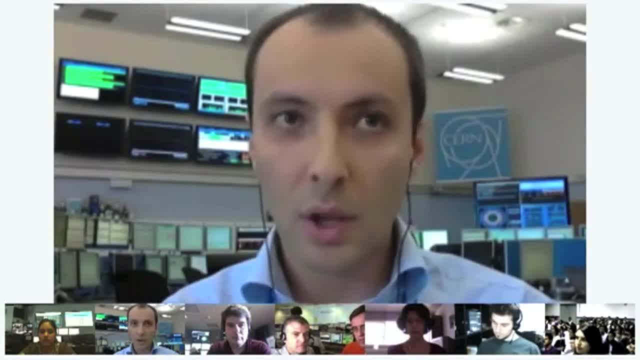 that made them to turn in a circle constant. so you will have to increase the diameter of your machine. or if you want to keep them confined in the same machine, you have to increase the magnetic field. let's say the size of the LHC was done such that 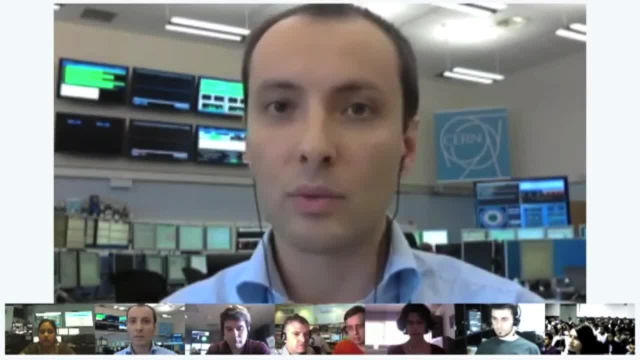 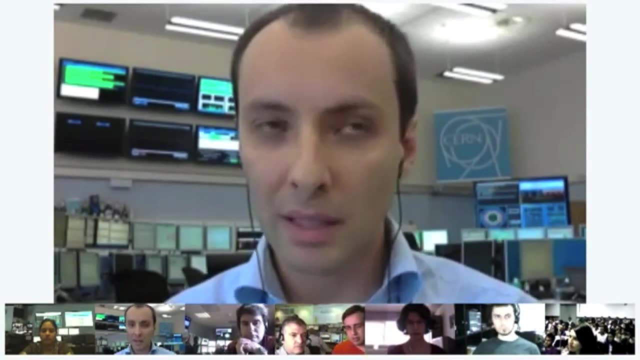 at the moment where the LHC tunnel was indeed the left tunnel. well, the tunnel where the previous accelerator was installed was chosen so that, with the maximum magnetic field which we could provide at the time, we could generate at the time with traditional magnets- we had the maximum energy with a 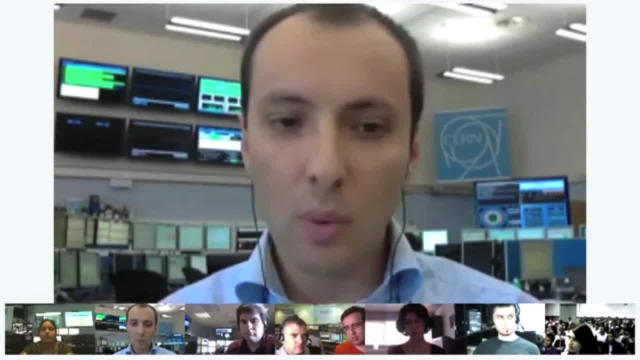 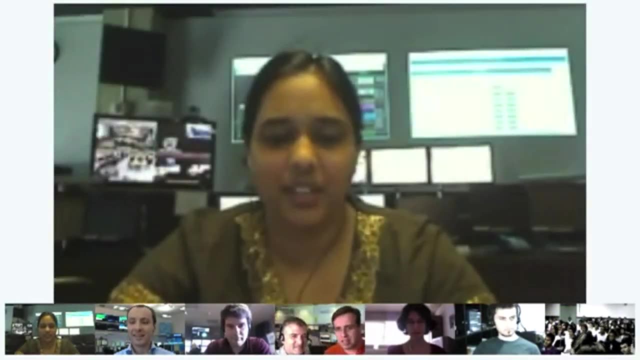 reasonable small machine. I don't know whether the explanation was complicated, whether you got part of it. So yeah, we really need very high energy particles and we need very high, very big machines to actually be able to detect them as precisely as possible. 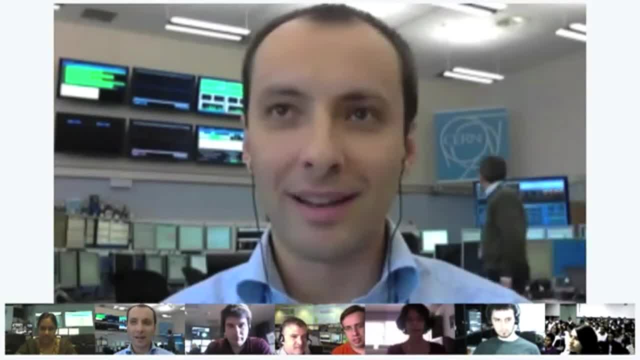 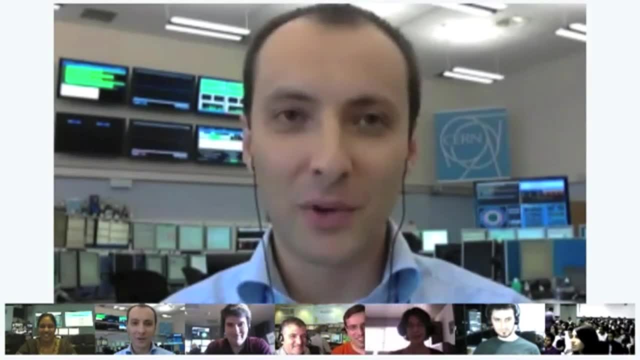 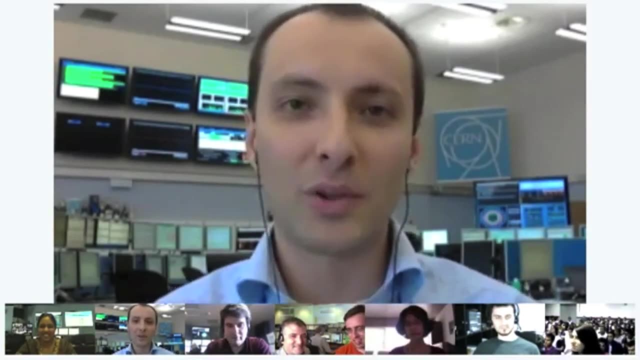 The ideal machine would be a thousand kilometer in circumference with the highest possible magnetic field, but of course both options goes against the. I mean both options need of course a lot of money to be to be used for that for the beginning. Okay, thank you very much. Thanks to all the three experts. 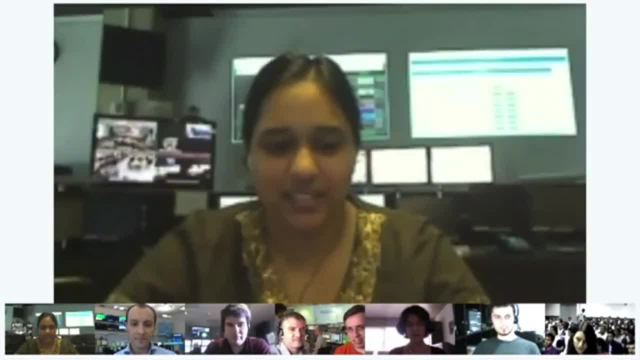 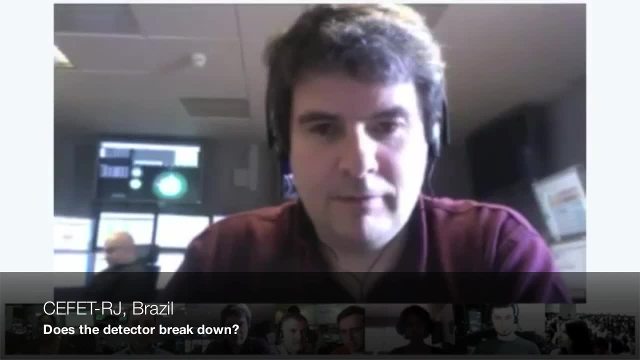 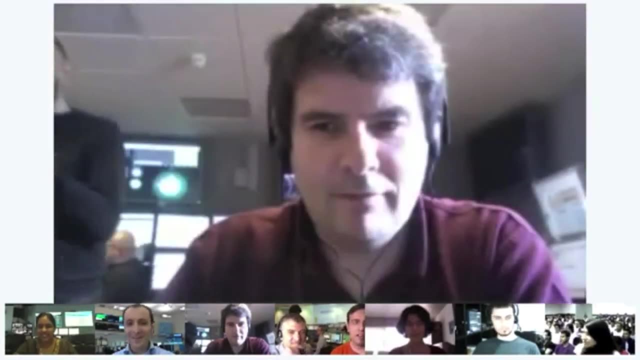 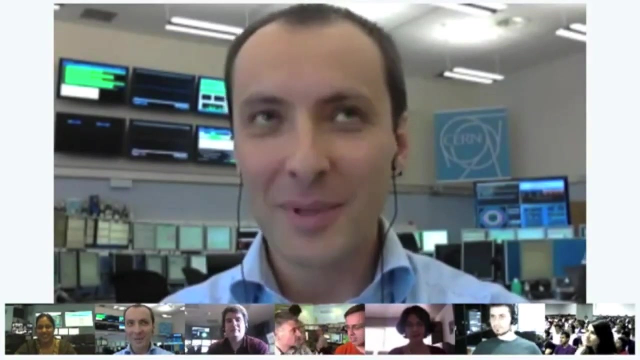 So should we go on to the next question: Does the detector break down? Ah, maybe this one. we will start with Marco. The question is: does the detector break down? Well, it's not me the right person to answer this question. I have in mind a clear. 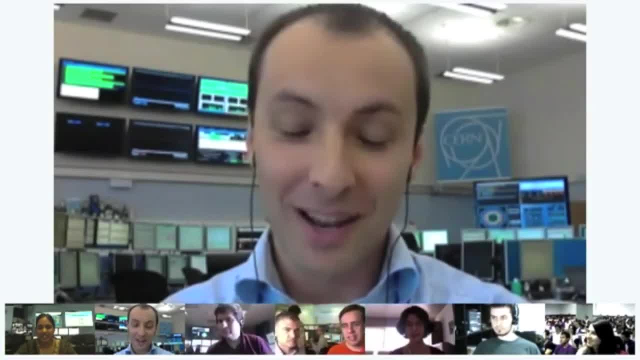 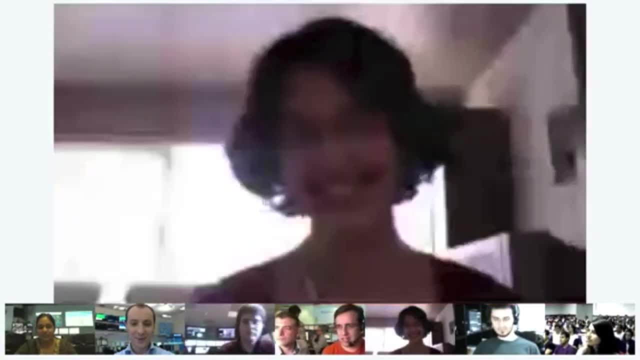 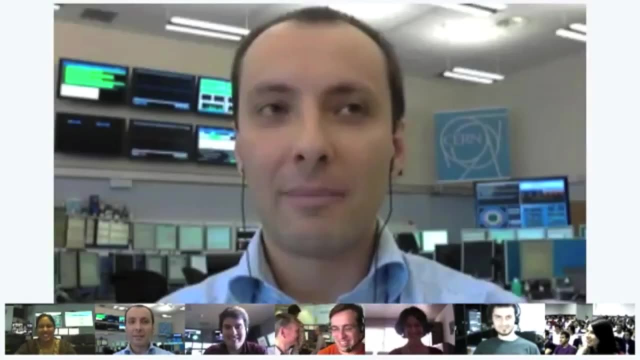 episode when part of the detector broke down broke down, actually It was a cooling part, a cooling element of CMS. Because of that, we have to stop the Hey, Hey, No saying bad things about CMS, come on Now. I mean I must say that 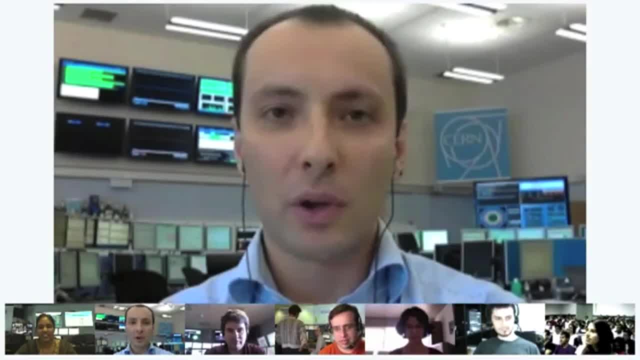 both the machine and the experiments are at the top of technology. They are very, very complicated elements. We have 27 kilometers actually of very high temperature, Very high technology components, So of course they, from time to time they that break down. 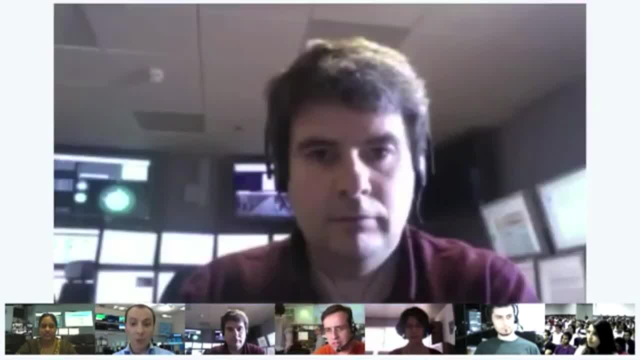 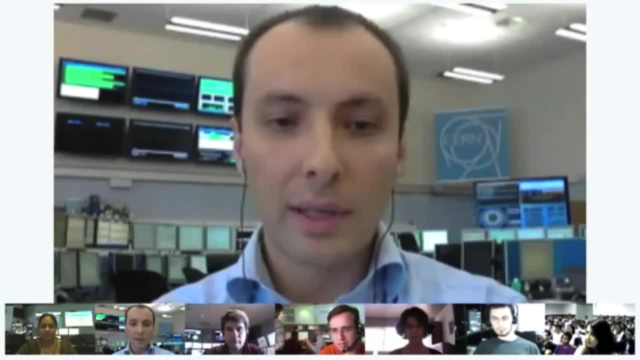 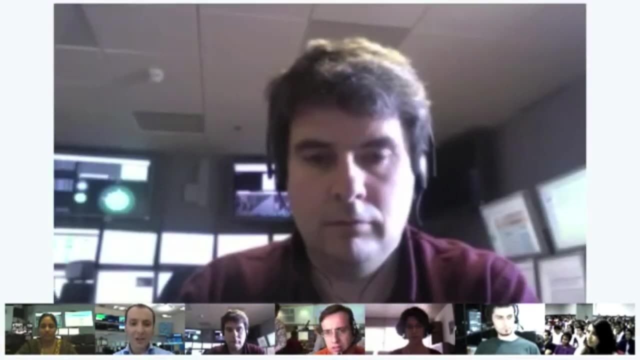 It happens for the LHC quite often, because we have more than 26 kilometers of magnets, electrical components and so on, Of course, the experience, experiments being, I think, less strong and less painful, big in dimension, they are enormous. 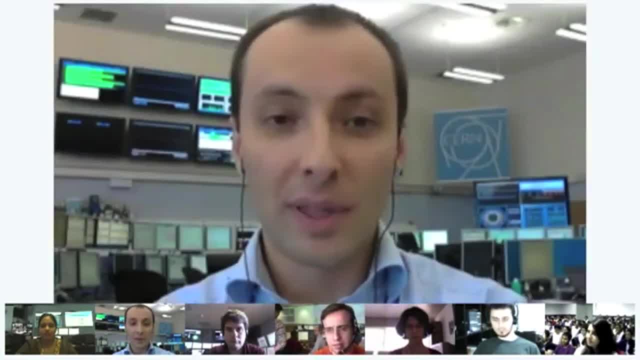 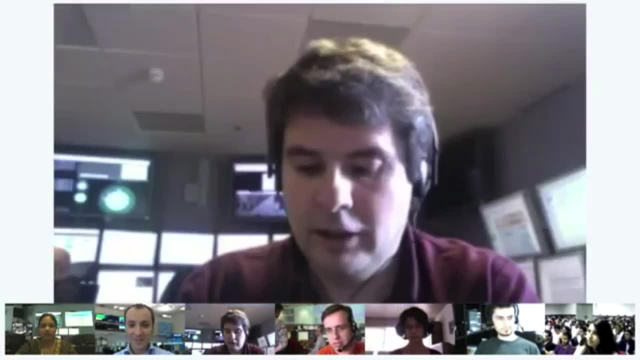 But compared to LHC they are smaller, Of course. the breakdown rate is, of course, low. I don't know, Dave, where the one comes from. Yeah, I can comment a little bit there. There's a big difference between the. 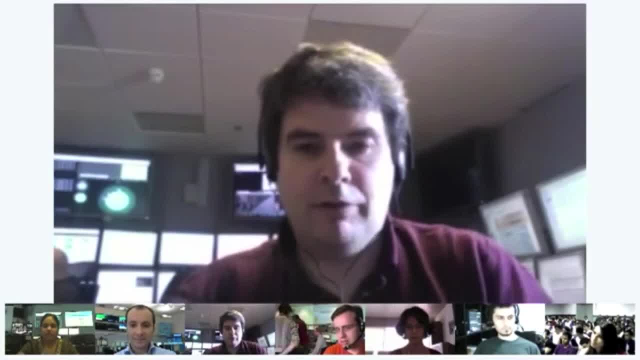 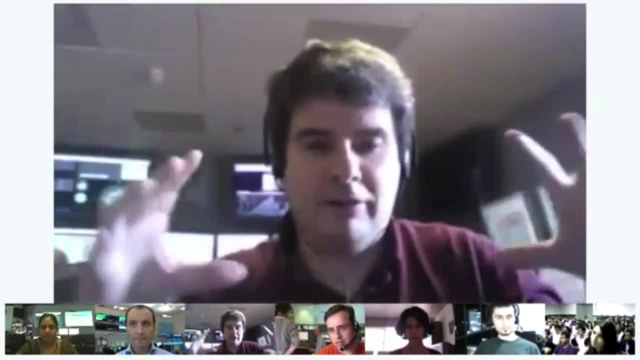 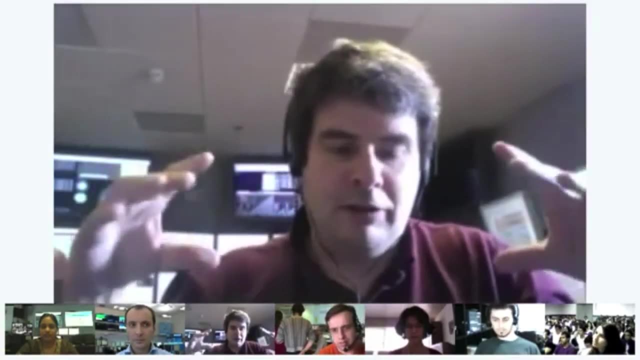 experiments and the LHC. What we have built for CMS, for example, is this enormous cylindrical object that has many layers, So it's a bit like a cylindrical onion, if you like, And each layer does something different- But actually accessing the inner layers of this detector. 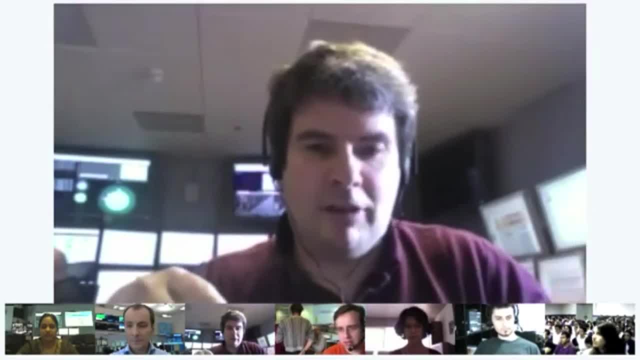 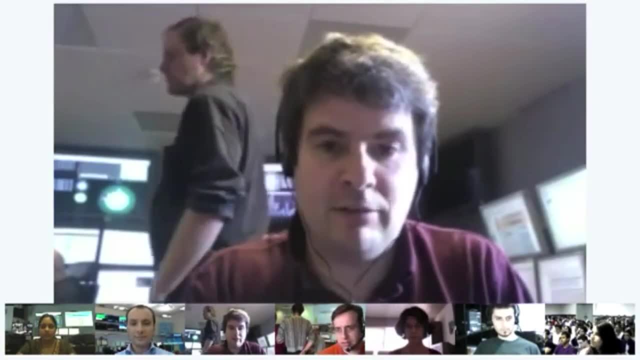 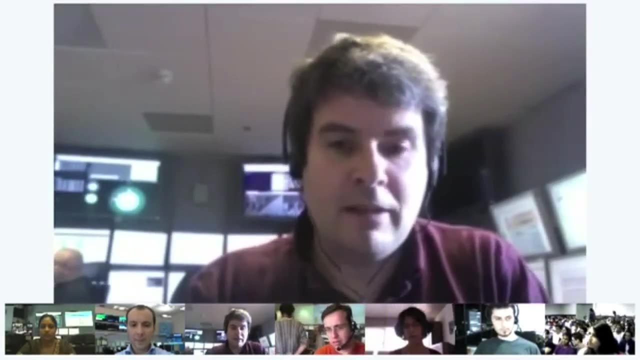 is really very difficult. So sometimes things do break, So they break really on the inside, But we have no way actually to access this. We have no way to fix these problems when they occur, So then we have to leave it. 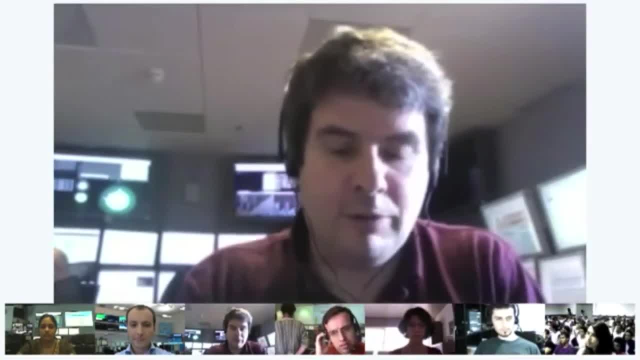 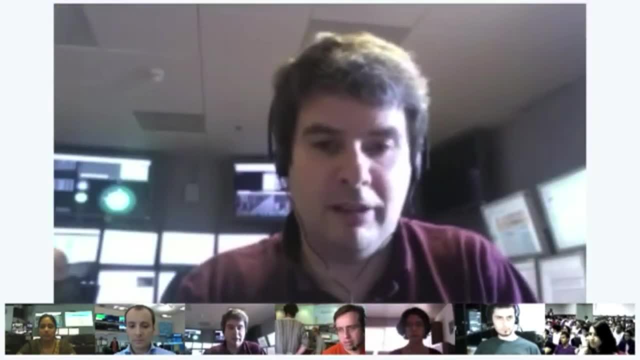 So of course we don't like that situation. So the way we build our detector is with what we call redundancy, So we have many layers doing similar things. So if one part breaks down, you've got the next layers that can take over the job. 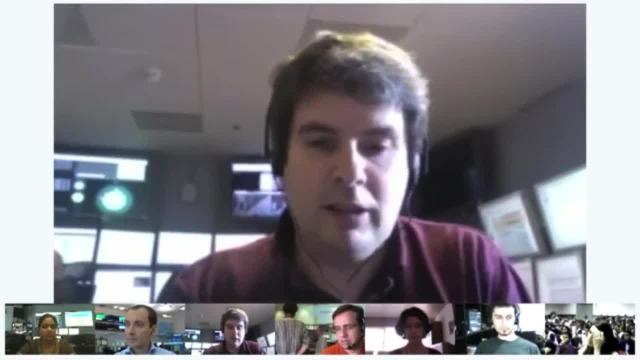 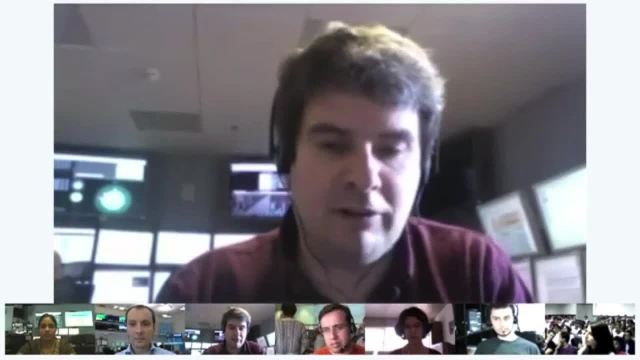 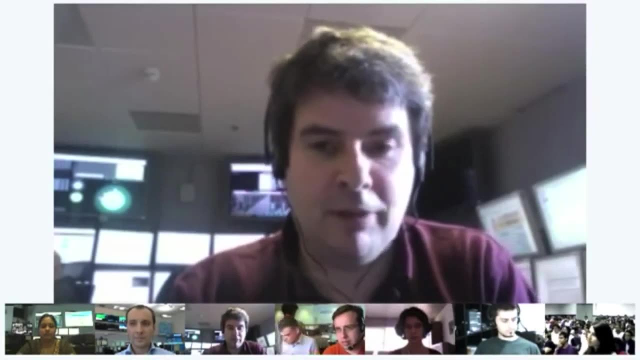 So even if some parts are not working, you can with the rest. At the moment in CMS, for example, we have about 99% of our detector is actually fully operational, And that's pretty good for something as big and as amazingly complex as CMS. 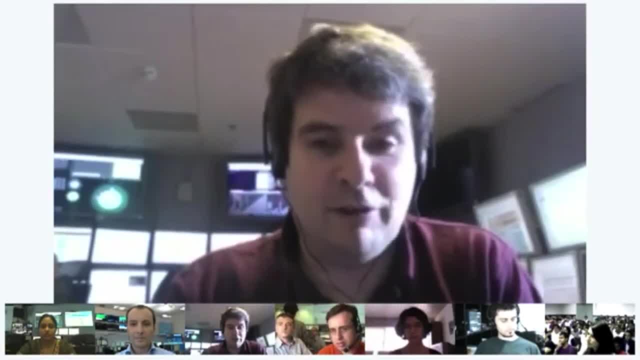 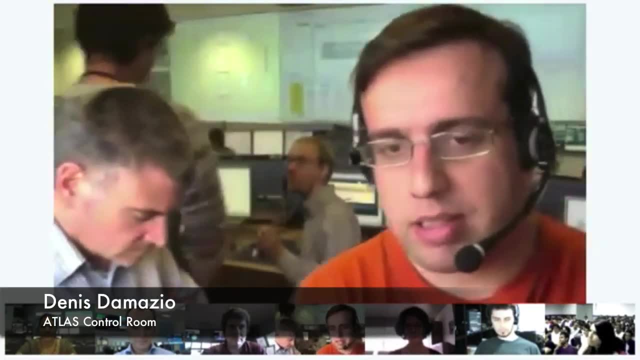 But of course things always do happen, but hopefully not too often. Well, if I can make a comment for Atlas, well, in the same way as CMS. so it's a huge detector, So the electronics that you have is quite complex. And the electronics that is exposed to a huge amount of radiation. so when you have the particles collide, you have a lot of flux of particles And this of course damages the electronics. So just to quote a few numbers, we have about 200,000. 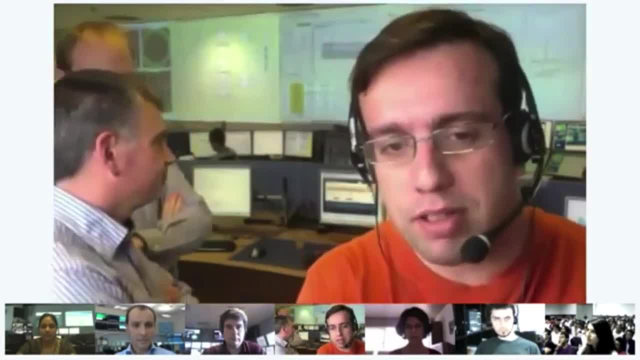 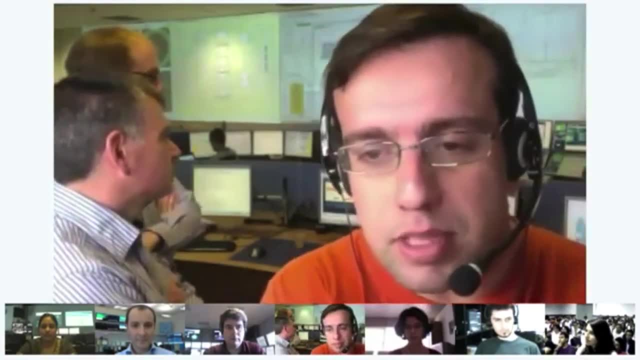 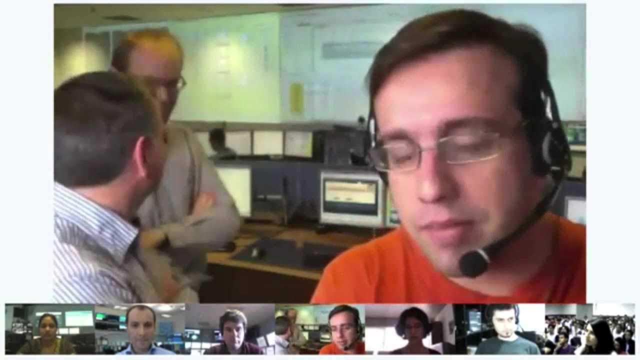 cells on our calorimeter, millions of pixels to be read out. I don't even know the number correctly. Actually it's a huge number. But the point is that it's a lot of electronics which is connected to the detector directly, So I can give you, for example, an example actually. 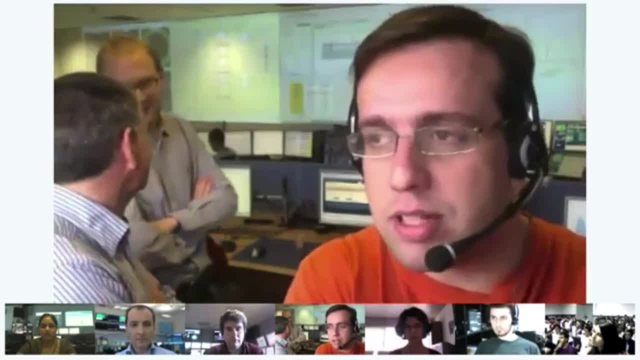 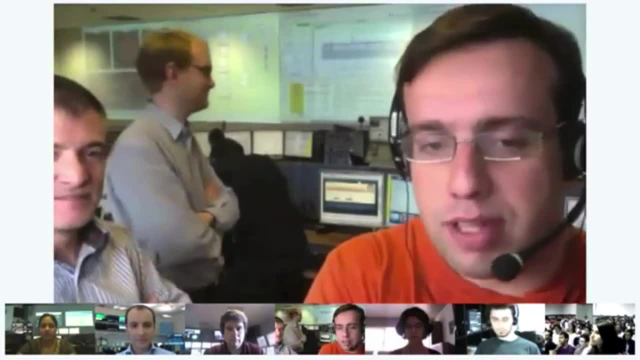 of the case For some parts of the detector that sometimes we have issues, like we have power supplies, for example, which sometimes may fail, And this, of course, is quite bad for Atlas. So what we do is we do exactly as the CMS colleague just 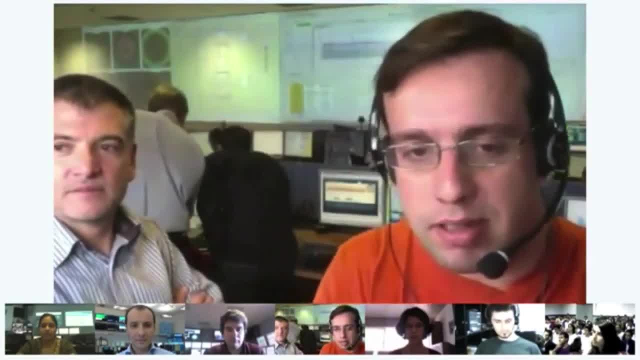 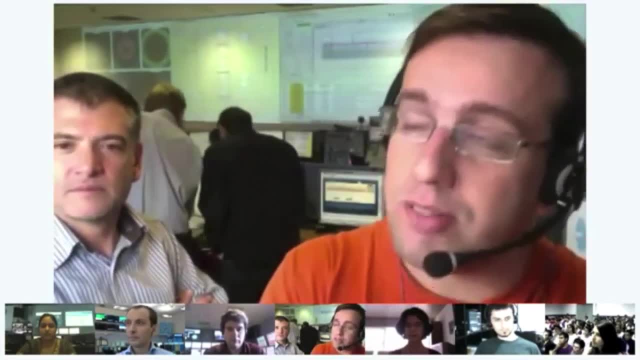 said, we have redundancy, So there are other pieces that take the job and don't let the detector stop working. But it's true that, for example, during shutdowns, it's not very easy to go into the detector, But eventually we can. 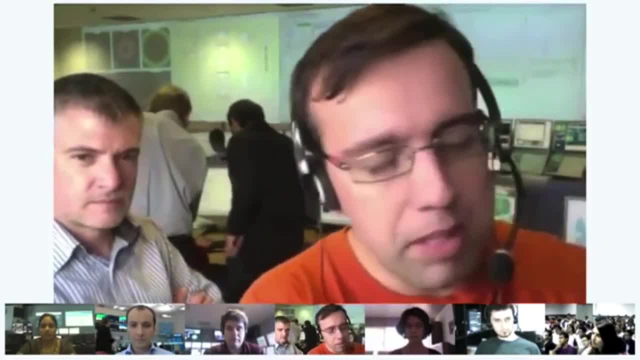 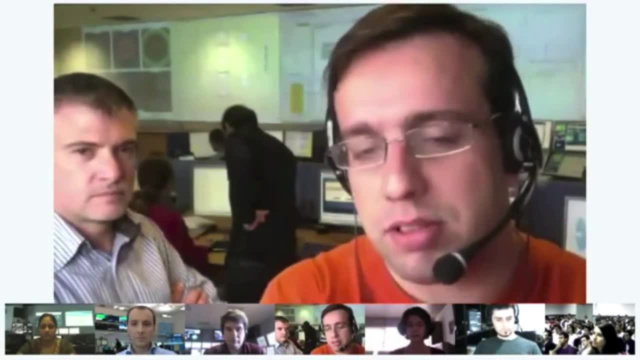 In some parts of the detector it can go, And, for example, at the end of last year, beginning of this year, during the shutdown period, I was actually downstairs changing pieces. So we do that from time to time. Well, you can only do that, of course, at the end of the year. 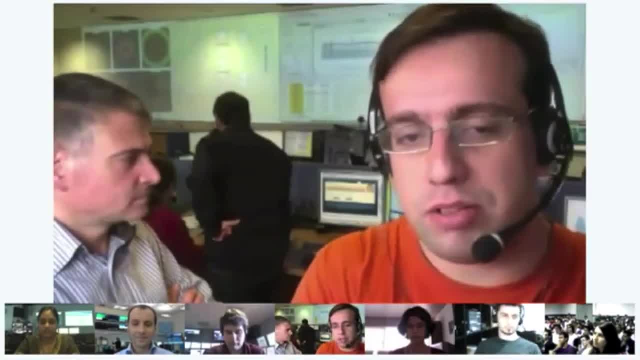 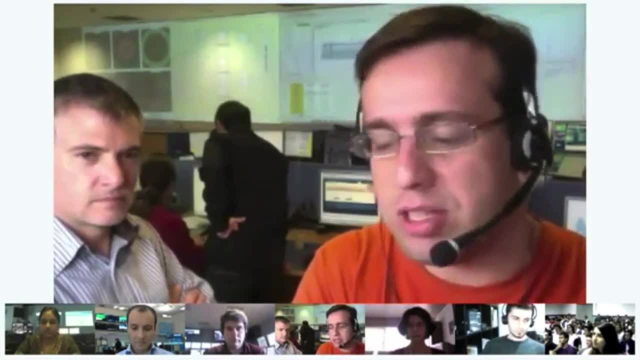 because we have to survive the full year doing data taking. We should not stop the data taking, But at some point we might just want to when we have the stop for winter shutdowns or Christmas and so on. some people do not have Christmas. 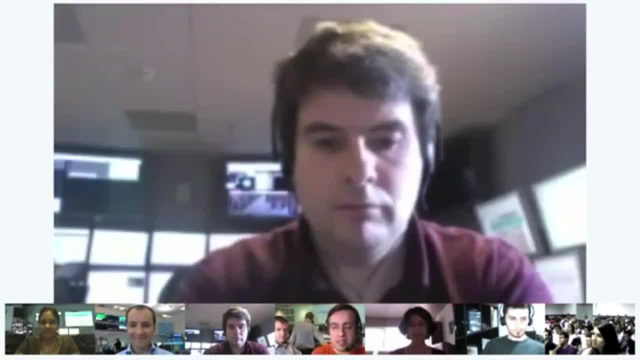 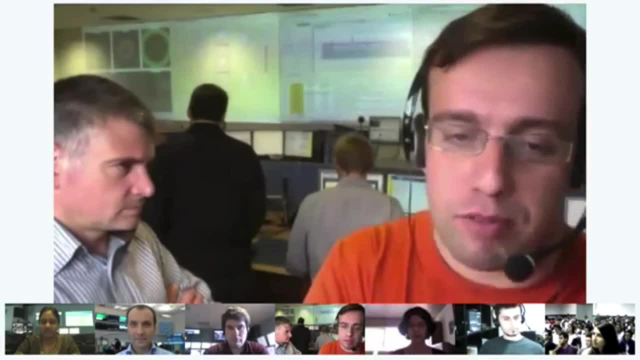 And some people go down the detector and try to exchange a few of the pieces that were That are not so good as the other ones. So this happens a lot And we have to have one safety thing, which is to have redundance. 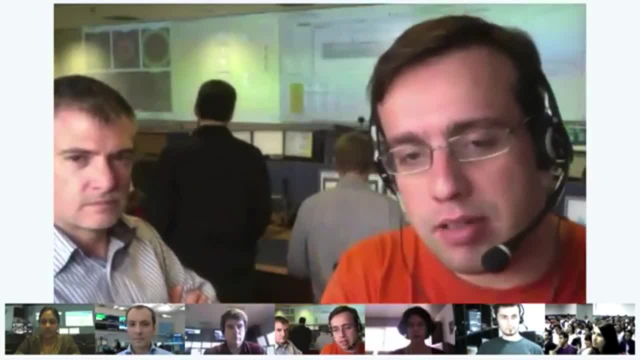 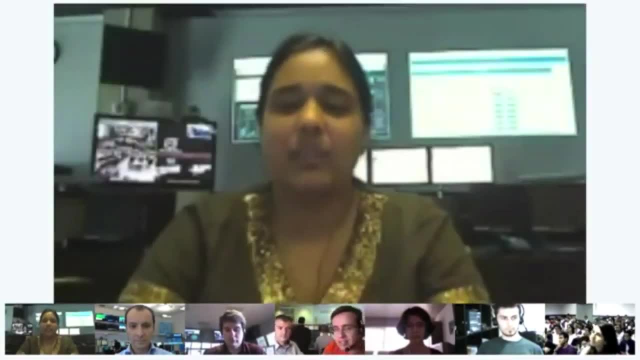 The other safety thing is to be able to, at the end of the year, go there and put the best pieces in place. And also I can assure you that there are a lot of physicists who have sleepless nights when you turn the detector on and off. 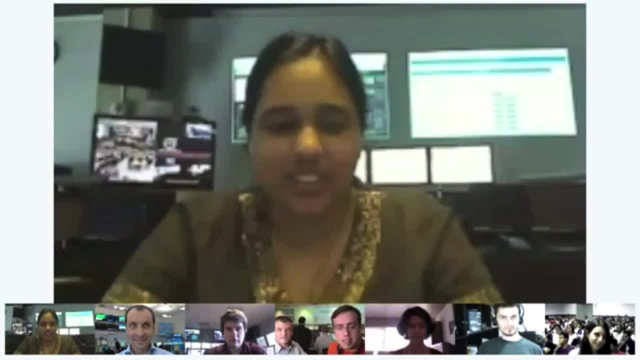 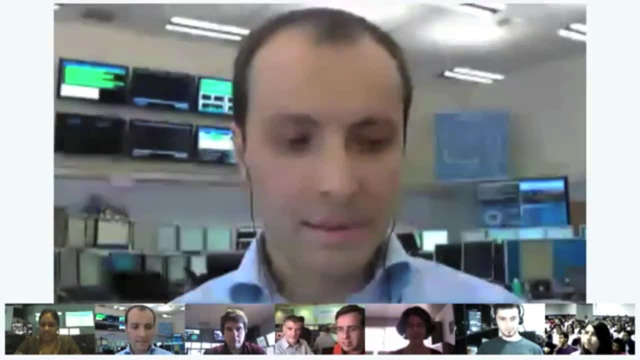 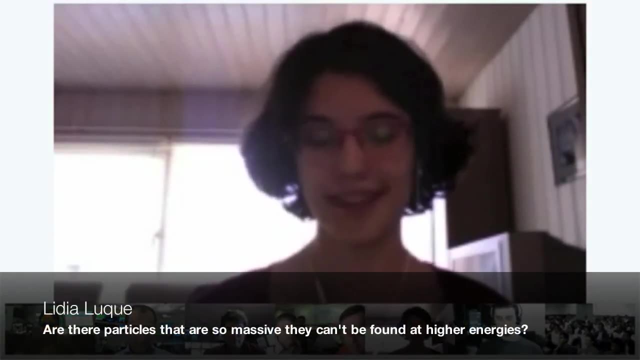 So, OK, thanks again to all the experts And also thanks to the questions. Now I think I will ask Lydia to ask the next question. OK, So my question is: is it possible that there is particles that are so massive that you're not going to find? 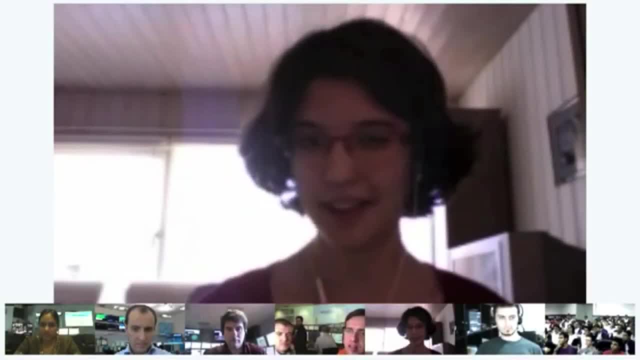 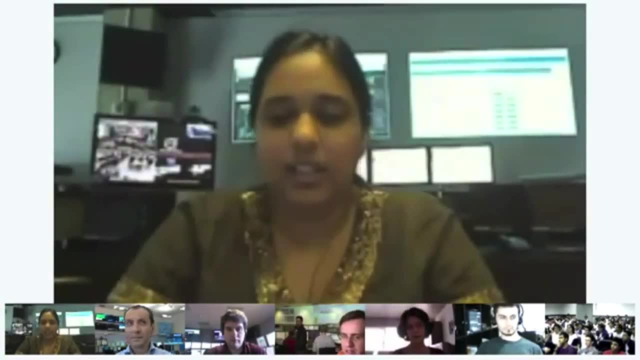 even at high energies, Like I don't know if it was 14 teravolts or something like that. That's a very good question. I mean, right now we are not running at 14 TeV, We are running at 8 TeV. 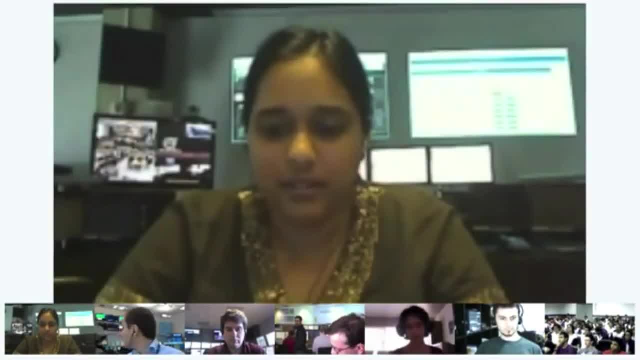 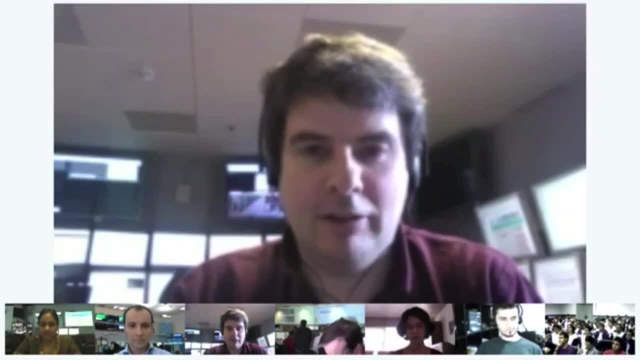 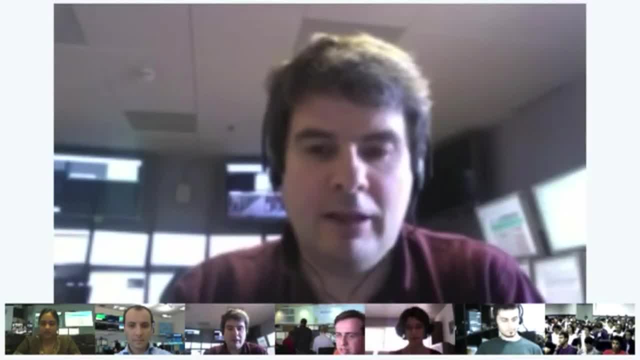 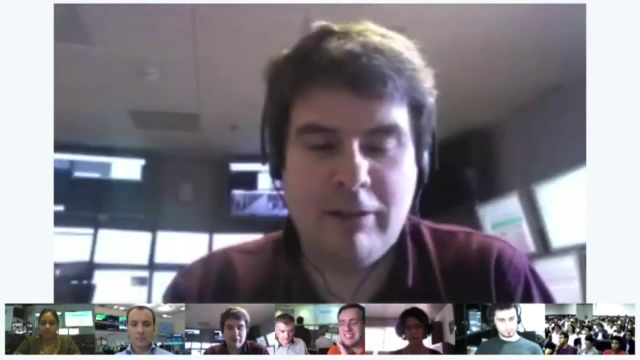 phenomena in the universe or another. Some of them are relatively light, like the Higgs boson- if it exists, is relatively light And we should find it this year. And even ATLAS might find it this year, which would be amazing. 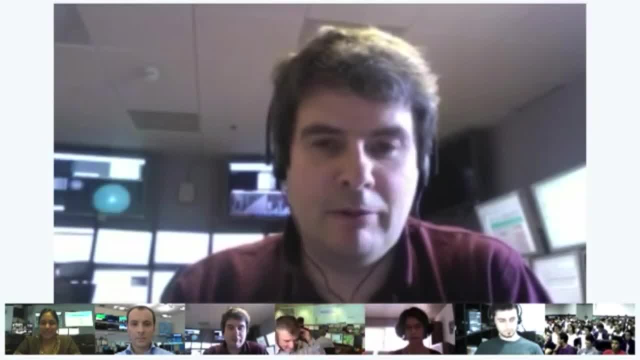 And then there are other types of particles that are, for example, heavy versions of some things that are familiar to us, like the Z boson. There might be a heavy version of the Z, which could give us indications of extra dimensions or many other types. 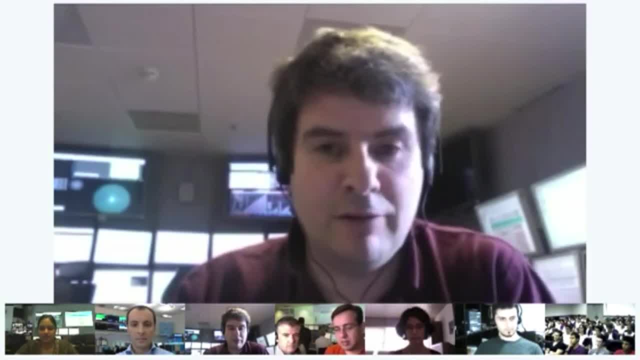 of theory And they may be much heavier, 1 to 2 TeV for example. So the LHC could definitely find those as well. But there may be even other theories that plus, you know, postulate much higher mass particles that clearly the LHC 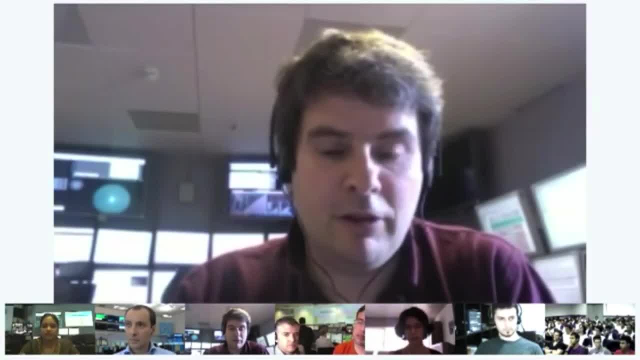 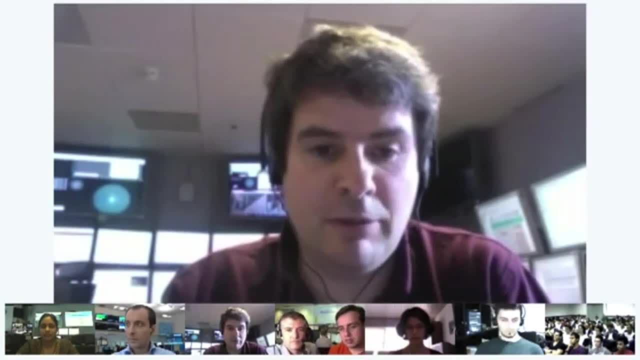 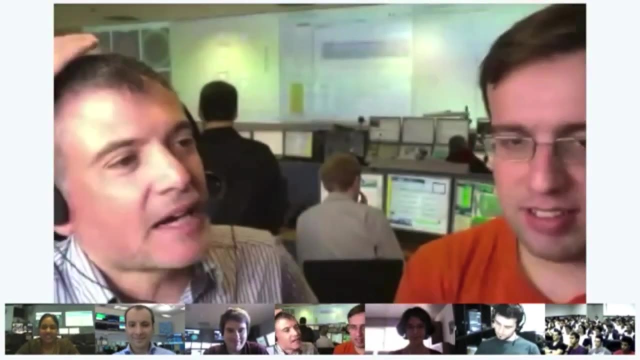 has a limitation And we won't reach those. I don't actually know what those theories might be. actually, that postulate even heavier things. So maybe Steve, my all-knowing partner on the other side of Ring, knows this Well. I wouldn't know. 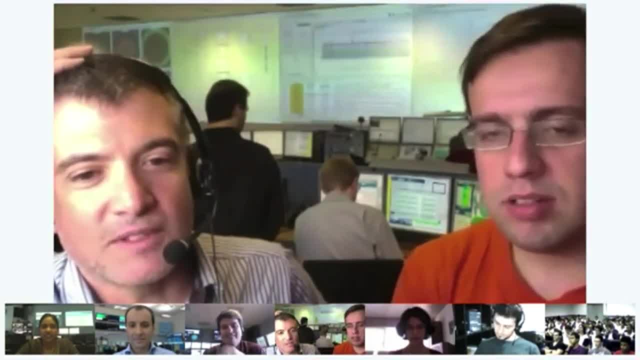 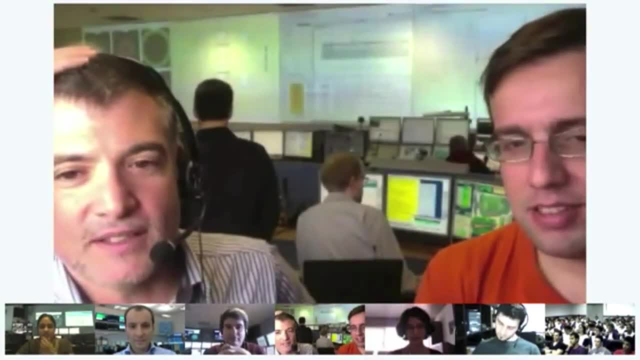 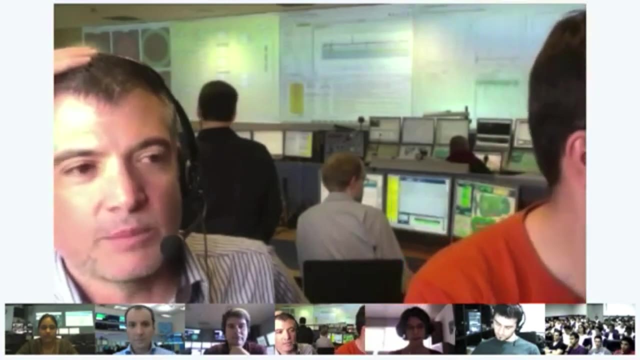 But what I would say is that I would give you an idea of the accounting that we have so far. So I'll give you our ignorance factor. What we know by looking out at galaxies is that, given the particles we know and that we have been able to measure, we 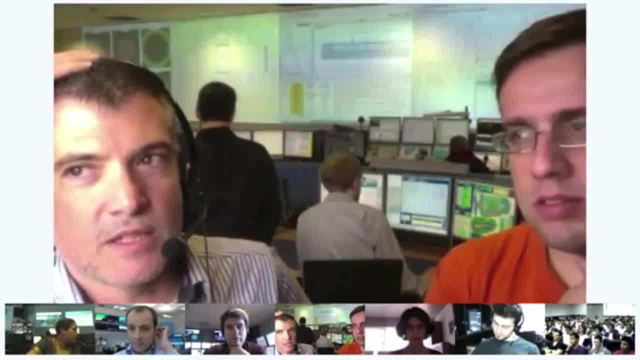 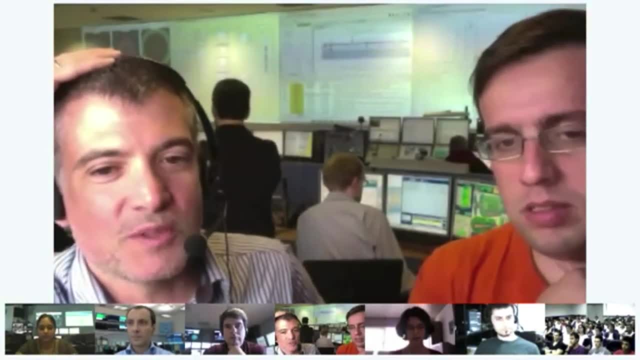 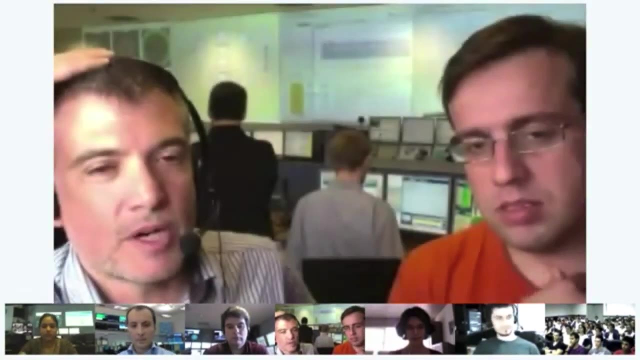 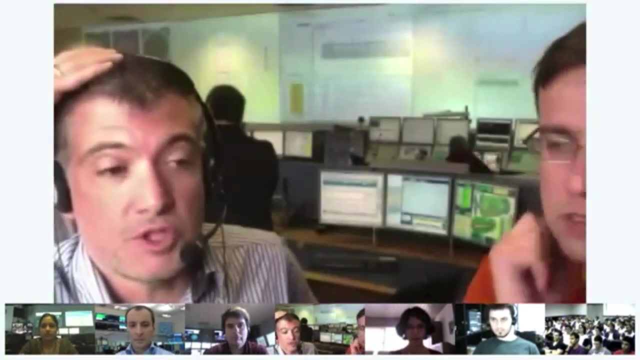 can account for about 20% of the mass that would be necessary to hold them together. So we're certainly missing a lot. And OK, And whether that's due to a particle that we might detect later on this year even, or whether it's due to a whole. 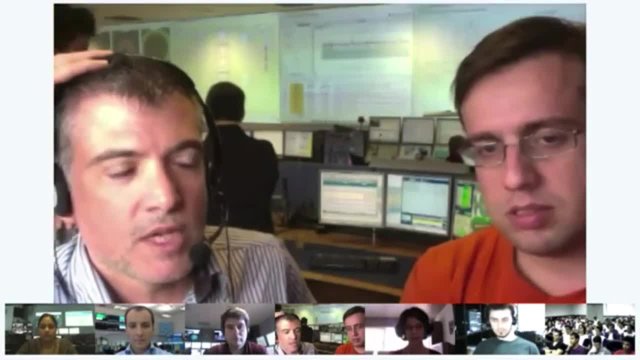 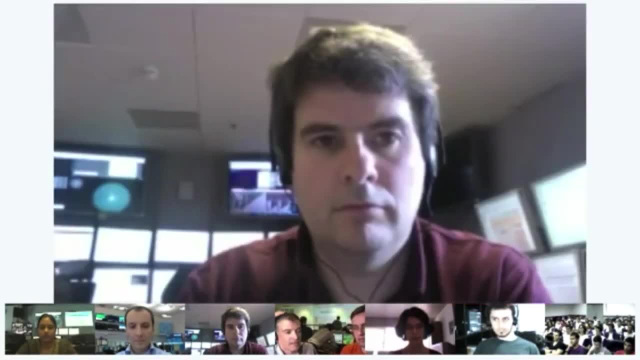 variety of different particles we don't know. Since we haven't been able to detect it so far, there's a good chance that even with the LHC, we'll miss it. And, by the way, these particles which we haven't yet detected, 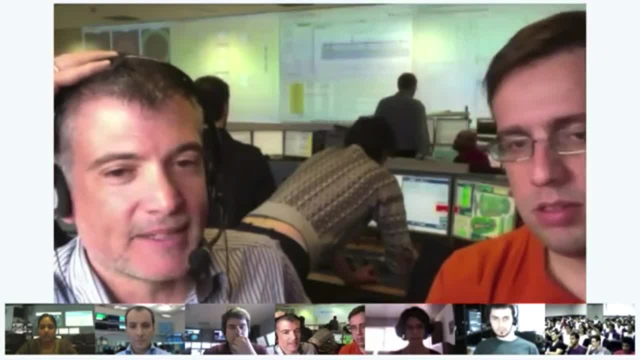 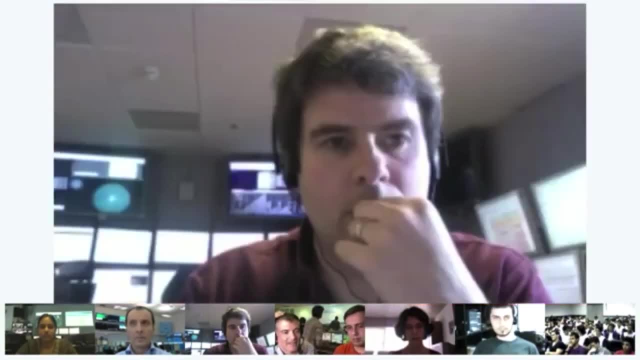 the way we look for them is by noting that there's an imbalance of energy when we have a collision and that something snuck out of our detector without us detecting it Statistically. we take a look at that and we will be able to. 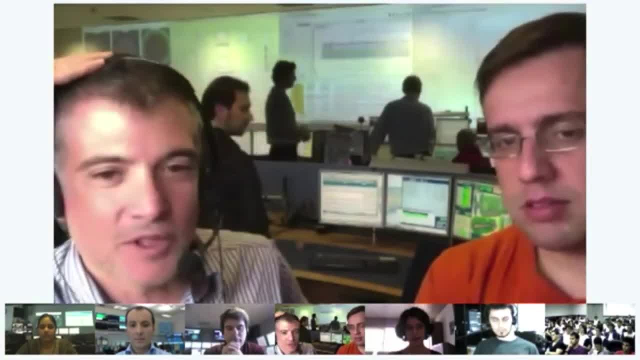 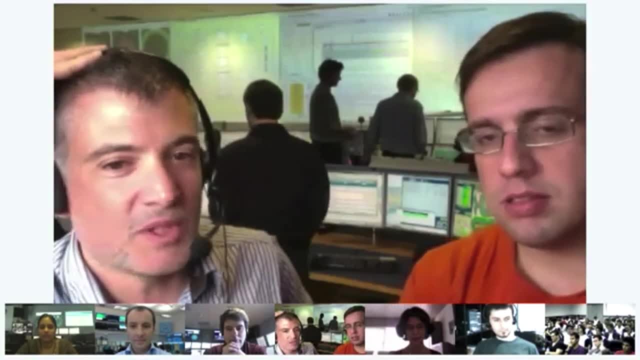 say something, But it's kind of interesting to know that 80% of what's out there could be something that we only see by noticing that we don't see it Right- Fantastic. So, yes, there are a lot of exciting stuff that we still 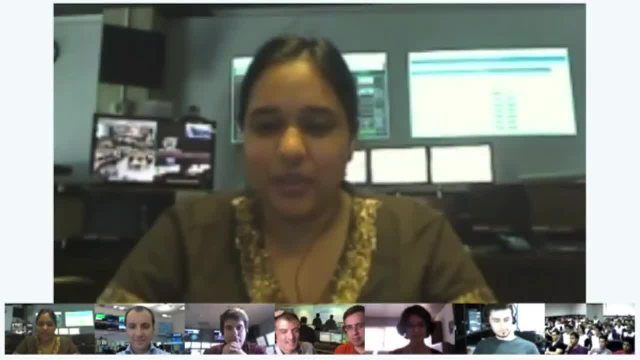 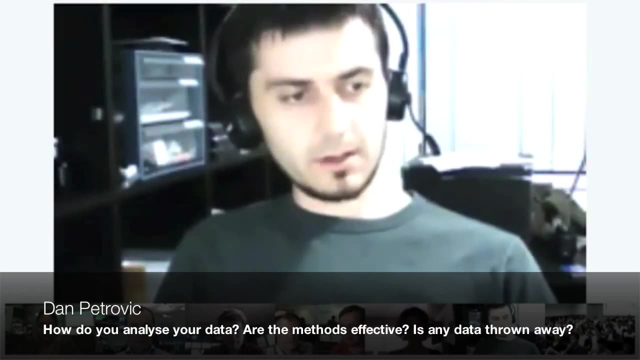 have to detect and we will look forward to it. So, given that we only have five more minutes left for this Hangout, I will ask Don to ask his question before we go back to the other game. Thanks very much. So my question is around the data and the way you handle. 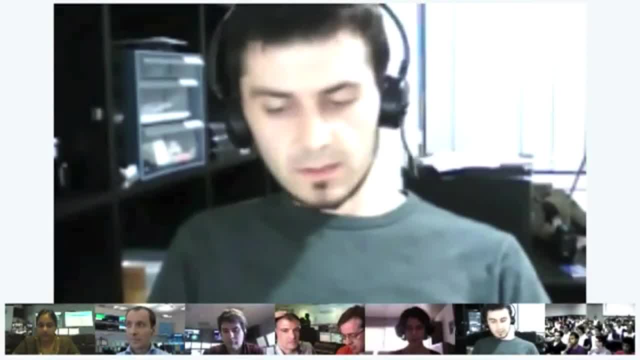 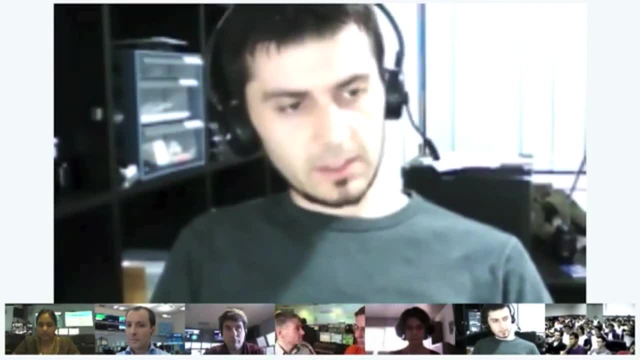 your data processing. One thing that puzzles me is the sheer amount of data that you collect through your experiments. If you could share with us just a little bit more about how you handle the data collection storage processing. Do you consider your data analysis methods and? 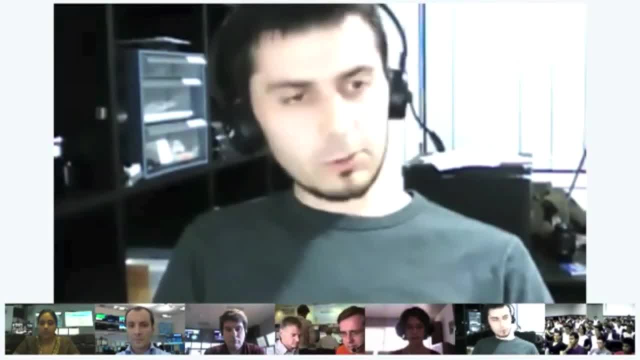 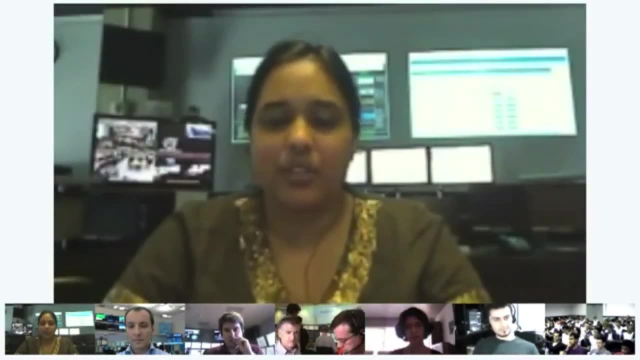 algorithms to be effective? And how long do you store all the raw scientific data do you collect? Do you at any point dispose of it? Are there any potential risks in doing so? Right, That's actually a very interesting and an important question that a lot of computer scientists are also. 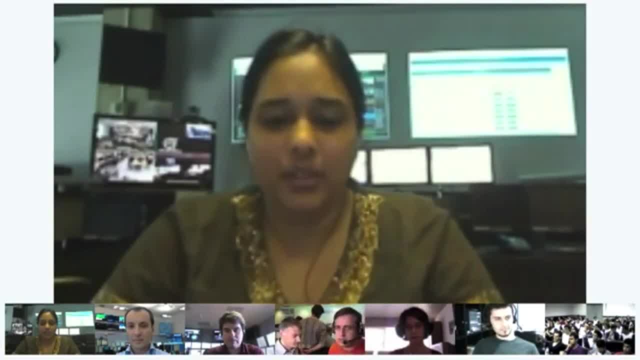 involved in trying to maintain our data. So I will first go to Atlas to understand their model and then maybe David can give a short summary of the CMS model and how we do it. They're more or less similar, but there are slight differences. 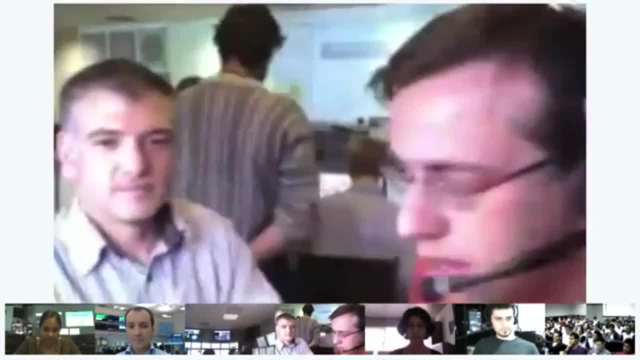 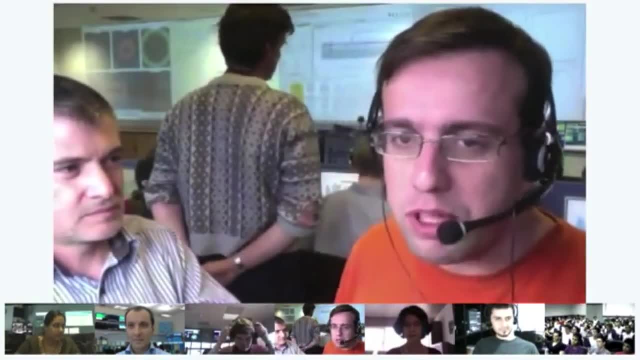 Atlas takes away. OK, So well. unfortunately we did not start to take data now, But if we had started, you would see that we can record up to 300, 400 events per second, And each event is more or less 1.6 megabytes. 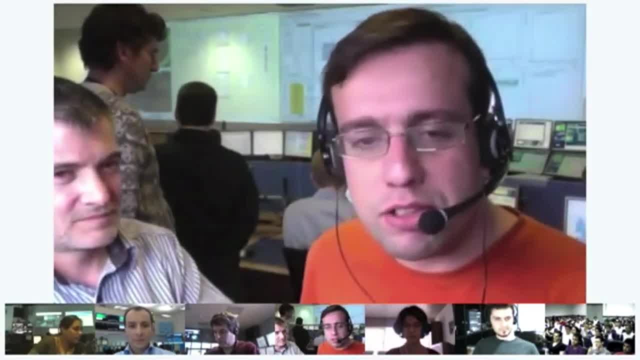 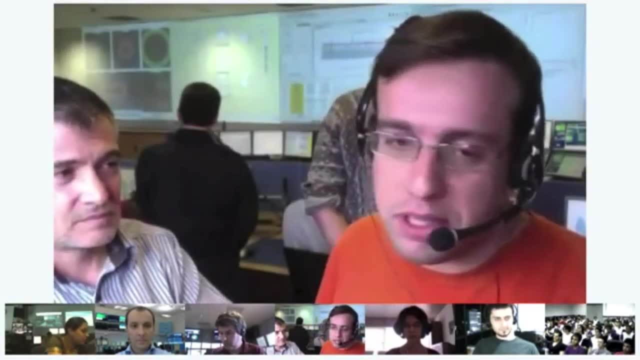 So if you start to make a count, I think you're going to see that you're filling a CD, a regular CD, every two seconds. So the amount of data is really huge And the amount of data that you take per year you can. guess it's a really huge amount. We have to not only store it somewhere and to maybe answer part of your question: we don't throw away. We don't want to throw away for as long as we can. at least so far, I don't think there's any plan of throwing. 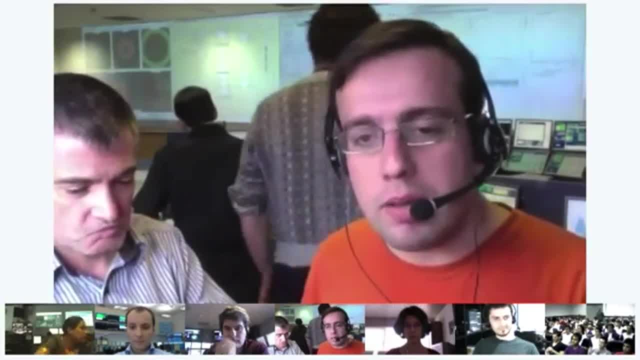 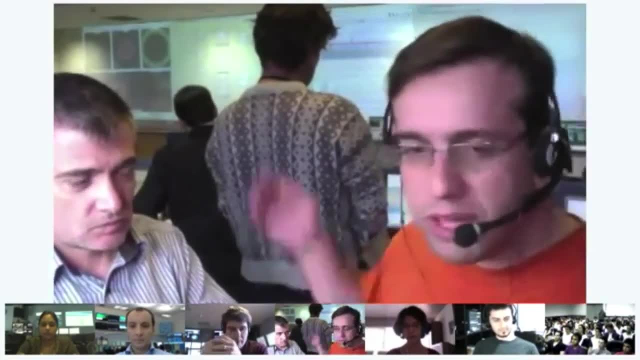 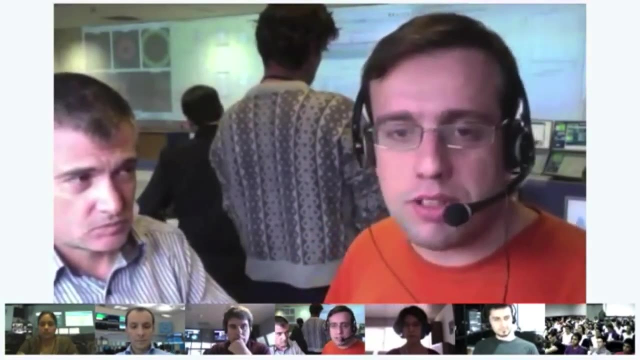 away physics data? not at all, But in order to also handle this data and try to extract physics OK. We also know that CERN, even though we have a computer facilities which I think has now more than 20,000 computers running there, this computer facility is not even 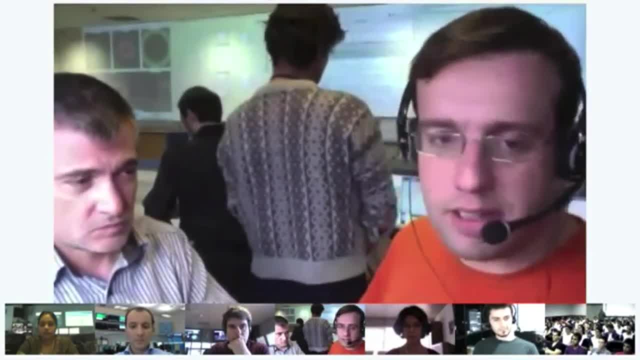 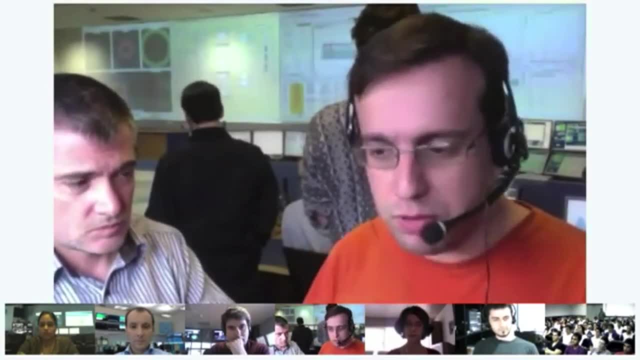 close to what is necessary to fully process and find things like the Higgs or whatever we're going to find during next year or so. So the way that we have in order to be able to really deal with this data is to spread data around all the world. 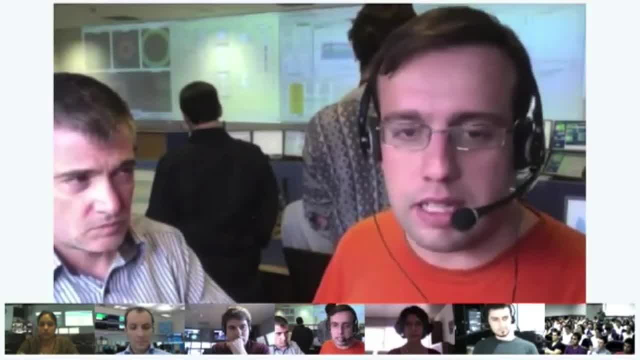 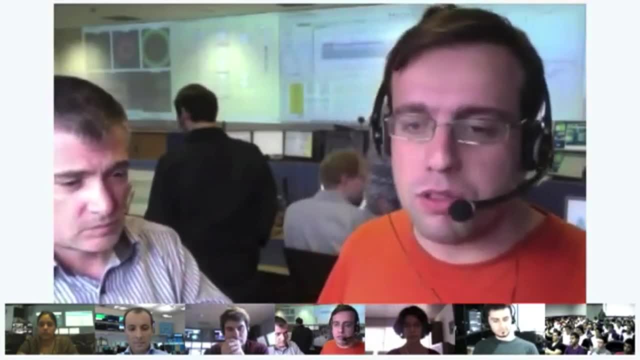 So actually we have 11 data computing centers- I think it's 11, right, 11 tier ones, as they are called for ATAS, spread all over the world. So there is one in the United States, one in Italy, one in. 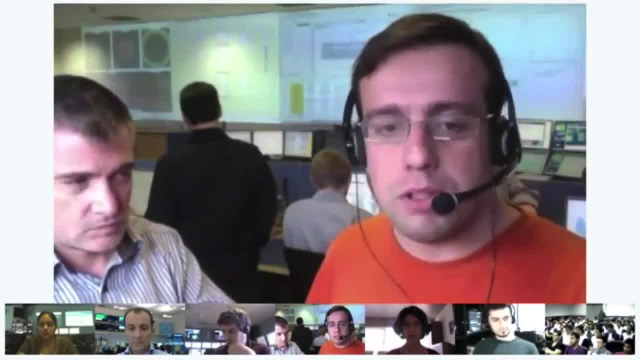 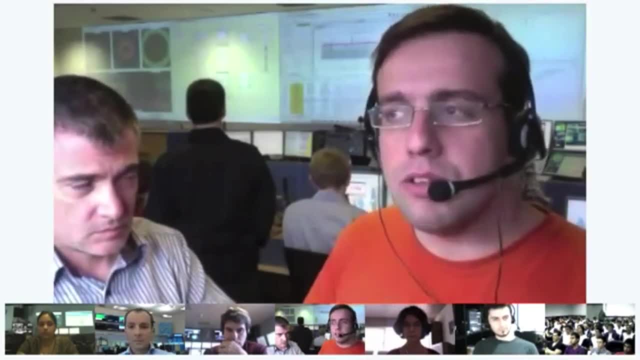 Germany, I think, one in France and so on, And we spread the data and we also spread the task. So the task must be handled at each place where the data is. And so then, OK, if you want to find a new particle or do. 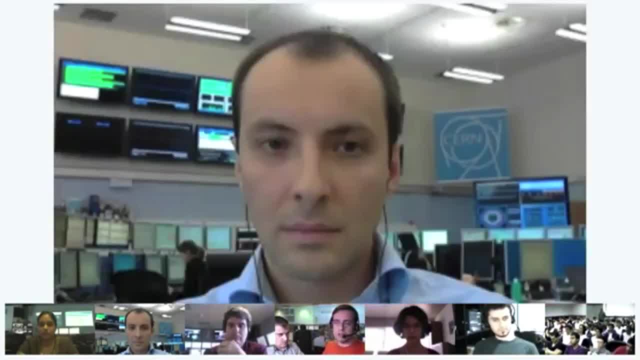 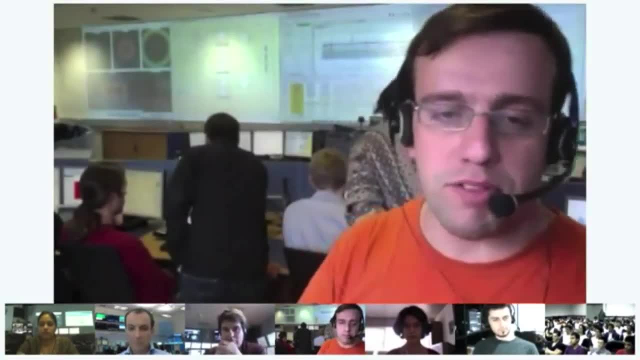 an exercise with all the data. you have to make sure that whatever you're going to do can be run in the same way All over the world at once, in such a way that at the end, you just get a small amount of data that represents your 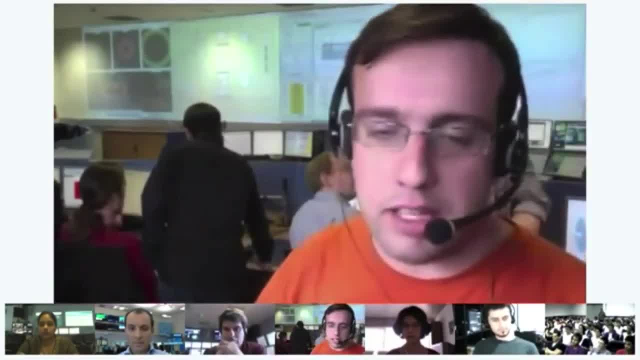 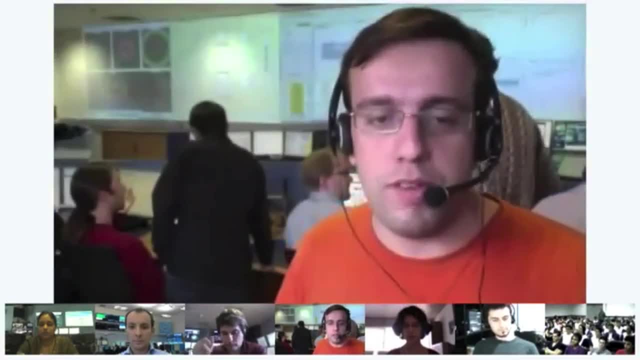 result that tells you that there it is. There is the Higgs boson, There is whatever your supersymmetric stuff, and so on. So that's the way that you have to make sure that you can run this in distributed mode and then afterwards. 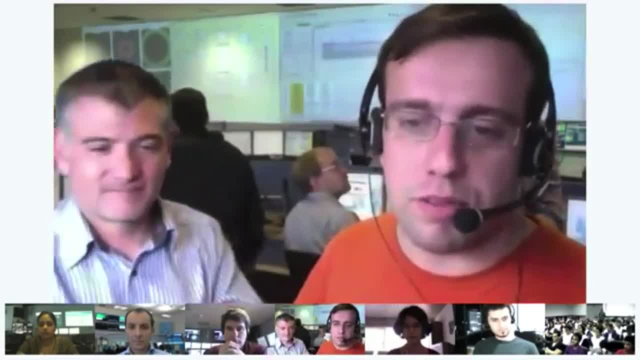 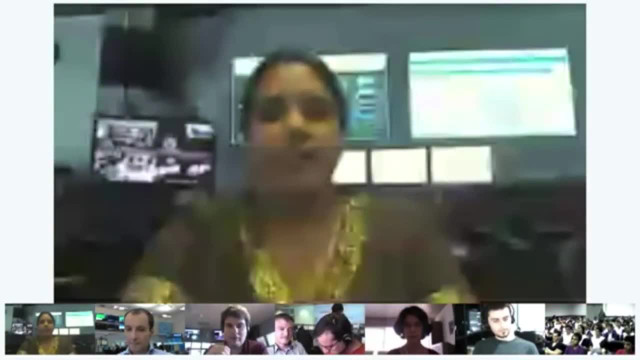 recover the data. I don't know if I mentioned the name GRID. This is what we call GRID computing. OK, yeah, So that's it. Thank you for the insight, And I think David can add a little bit more on how different is the CMS model. 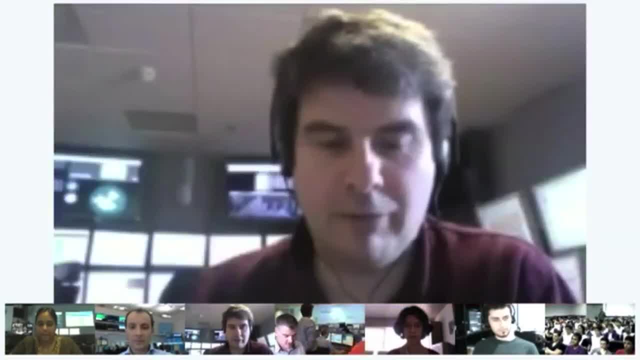 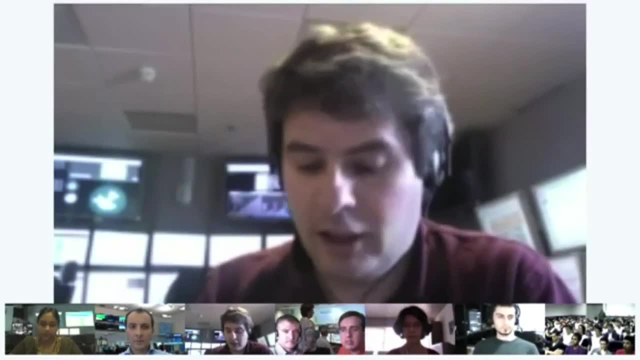 I mean, the CMS model is essentially the same, but I just wanted to go back a step to one of the parts of the question you asked about. do we throw away data? In fact, we throw away 99.999% of our data. 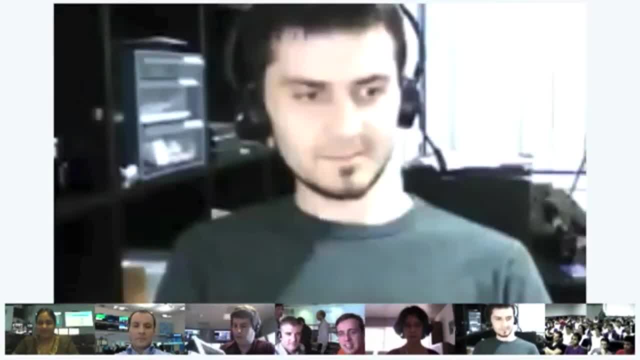 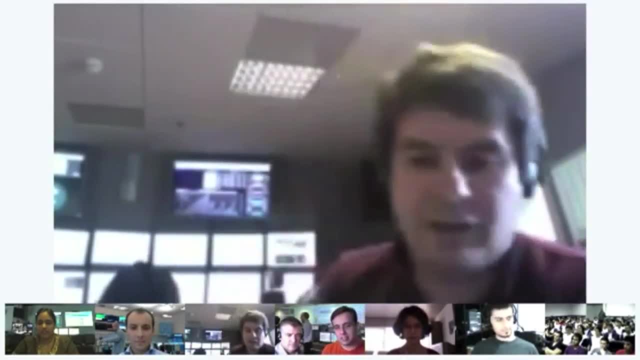 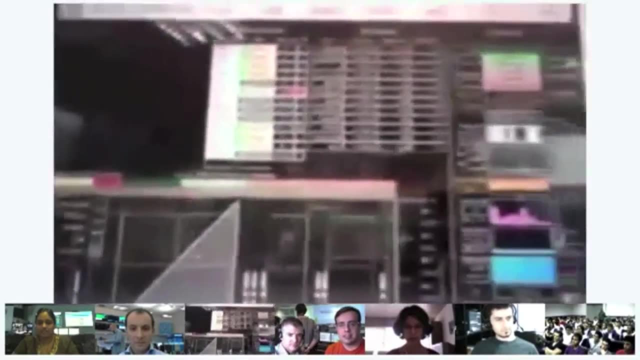 So let me show you. Let's see if you can see this. Actually, on one of the screens behind me there's a display of our data acquisition system, But I'll bring it close to you. Let's see if you can see this. 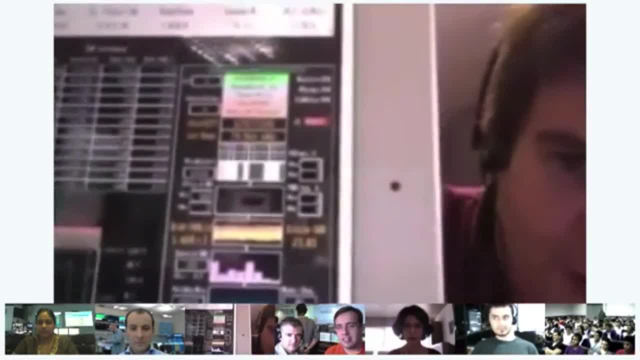 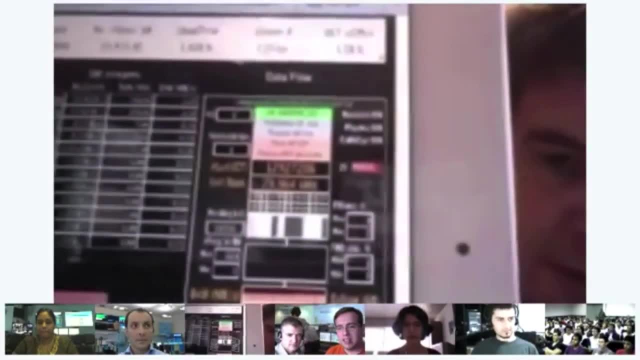 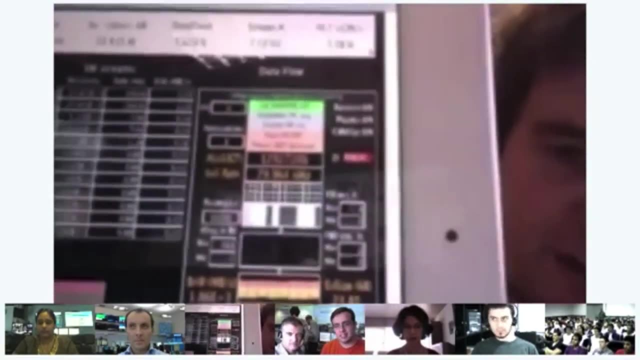 Not very well. So there's a number in there that's backwards, which is really helpful to you, which shows that at the moment we're taking about 80,000 events, or the equivalent of 80,000 collisions every second. Now, of course they're not. 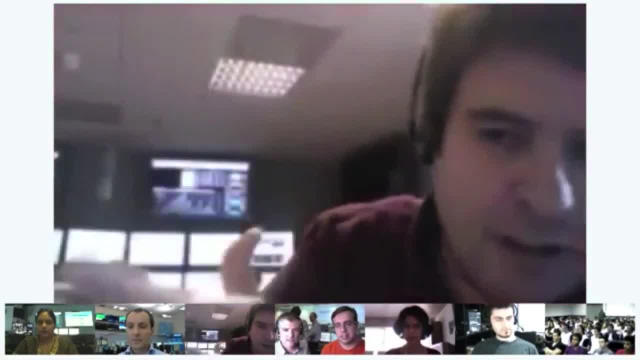 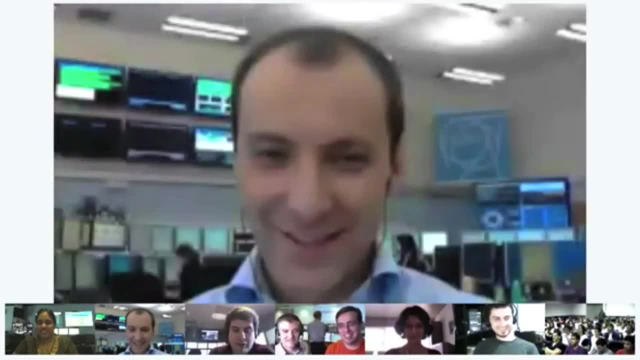 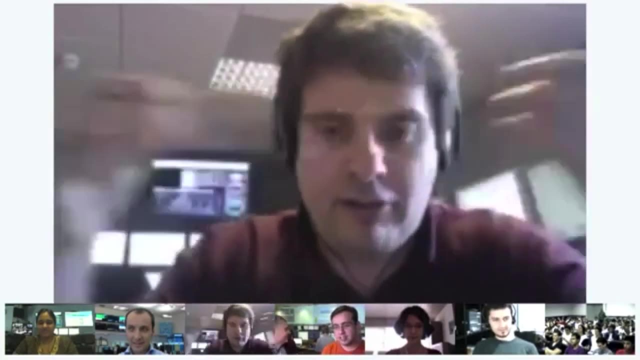 real collisions. at the moment We're still waiting for our LHC guys to do their job. One more dig at Mirko. But we're running at a very high rate. And what this rate is? we have all of these collisions happening all the time. 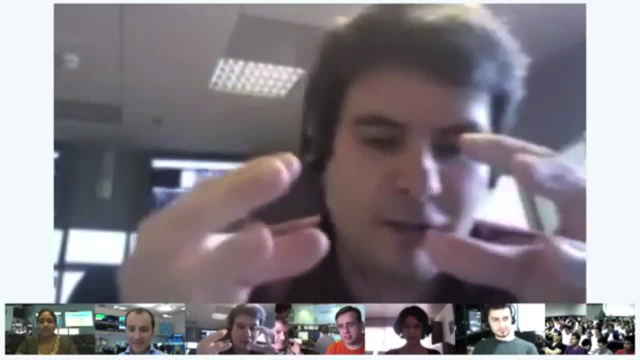 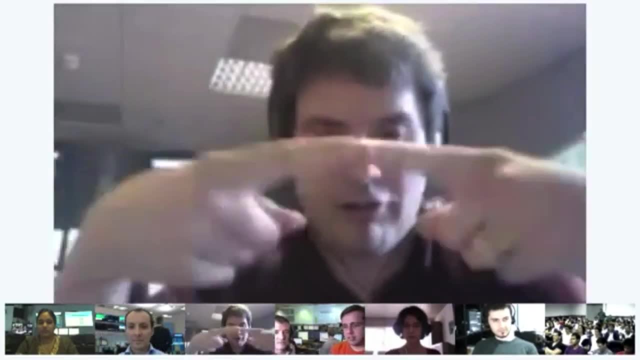 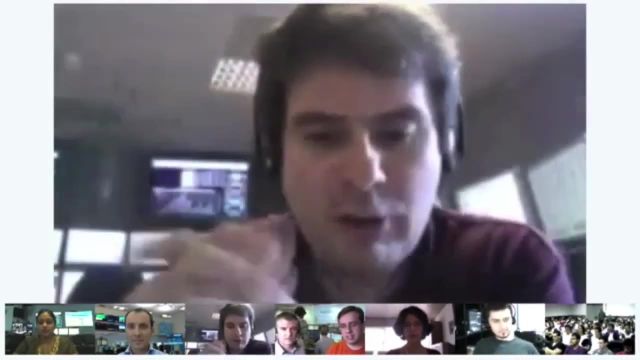 So we have about millions at the moment. I think it's going to be around 20 million collisions happening every second, or 20 million crossings of protons every second, And we have to take a very quick decision on which ones are actually of interest to us. 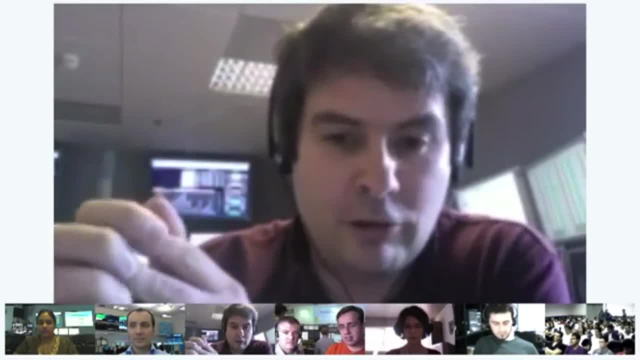 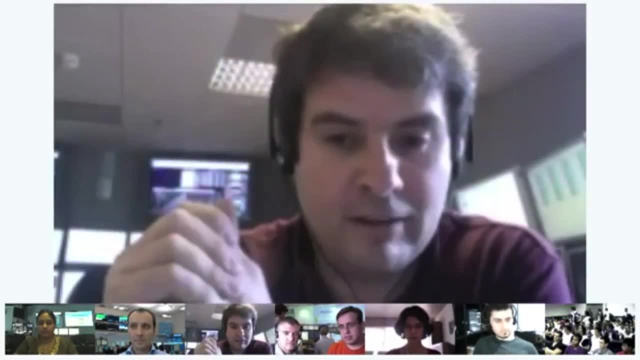 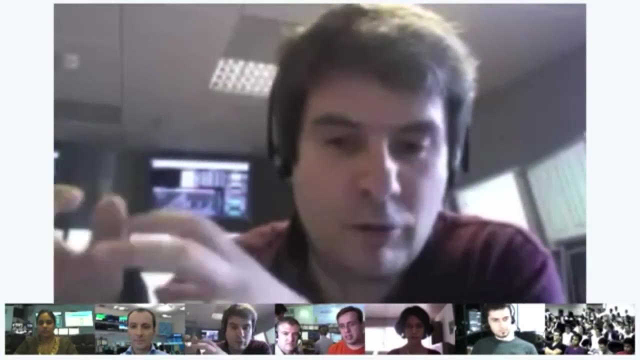 And, as Steve and his colleagues have said, we can only actually store a handful of those. like 200 to 300 of those collisions can we actually store every second. So most of the data we have to throw away. The number I showed you- the 80,000, is what's left out of. 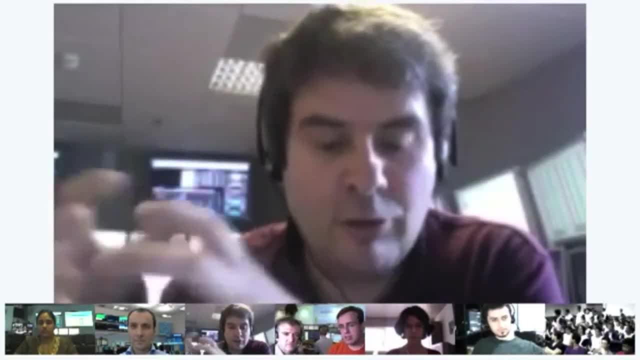 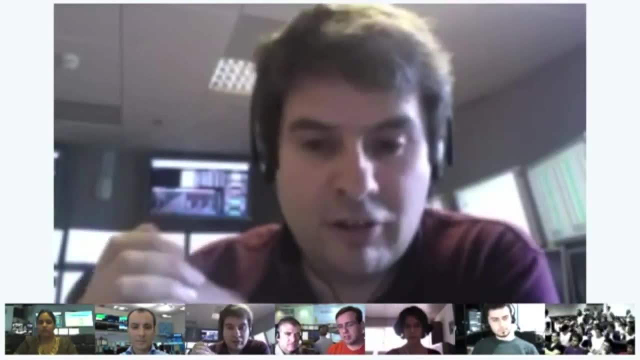 the data. But after we've made a first decision, we look at some basic characteristics of the data very quickly and try and understand whether it's interesting or not. Of course we have to be very sure that we take the right data and don't throw away all the good stuff. 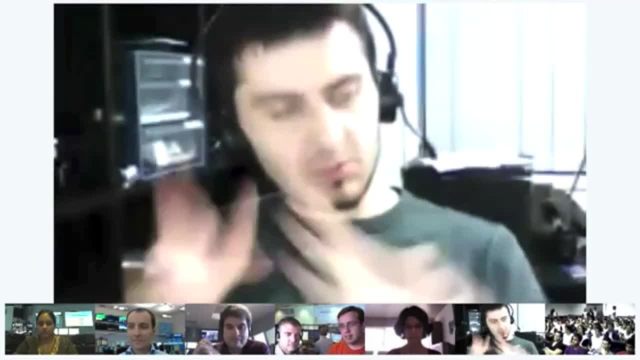 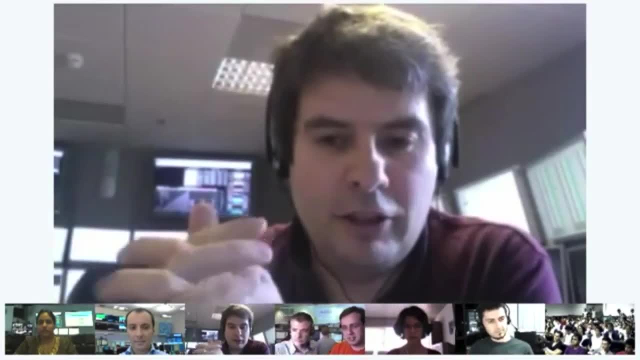 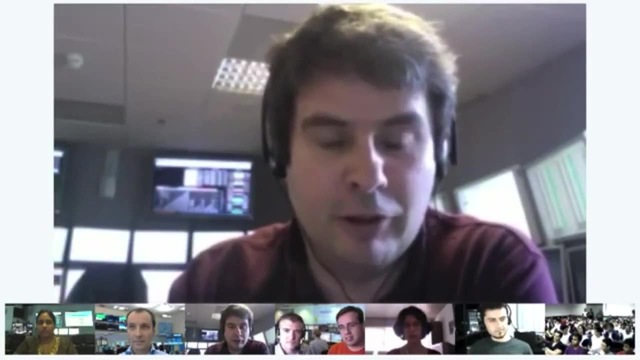 So you have an educated guess in the process, right? You decide which streams to ignore and which ones to record to save. Yeah, Imagine, you get all the newspapers in the world For a certain day And somewhere in there there's a story that you really want. 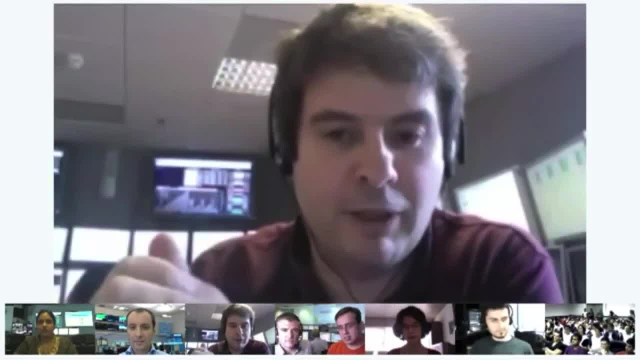 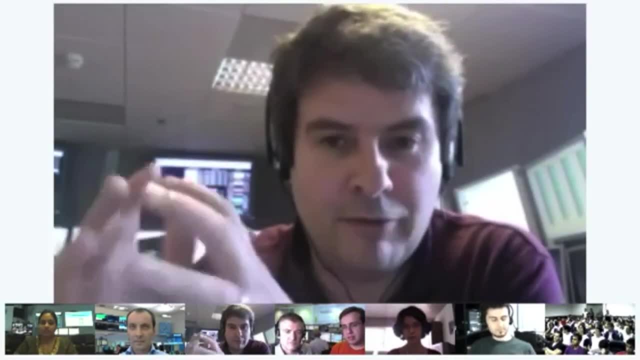 So the first thing you do is you know some basic things. You know the story might be in Portuguese, let's say. So the first thing you do is you throw away all of the newspapers that aren't in Portuguese. So you'd make a very brief, very quick decision, a very 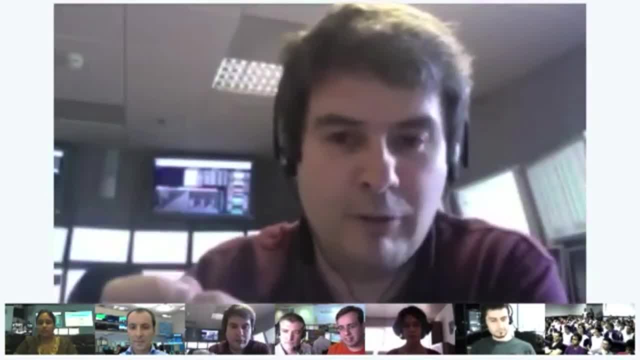 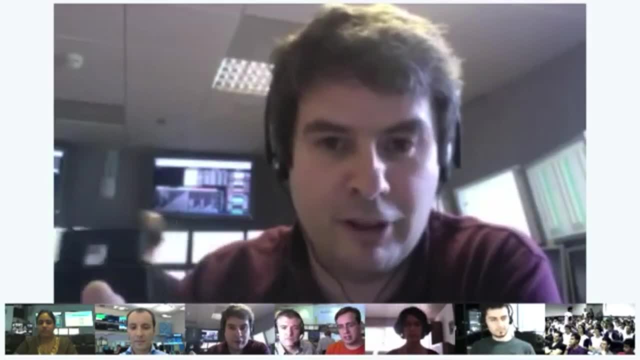 basic level. You keep something And now you look through all the Portuguese language newspapers and you look at the headlines. So that's your next step of filtering, If you like, And then, finally, you look at the headlines that actually concern you and go through those stories in detail. 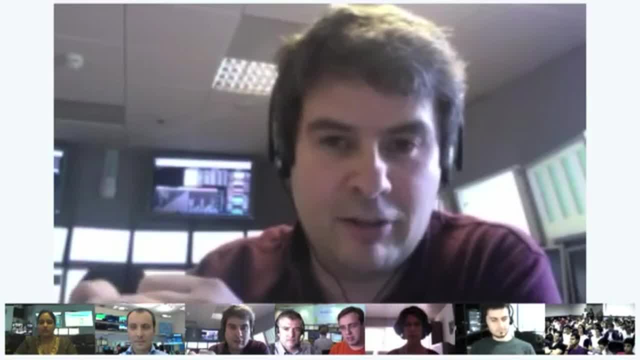 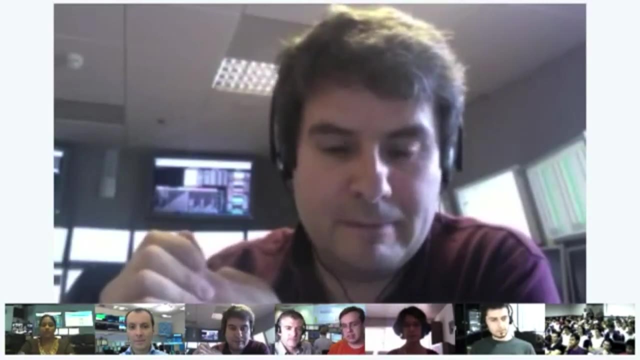 So we have these different levels that are very similar to that in CMS and Atlas. We make a quick decision on very basic things, keep some large fraction of the data, have a look at it in more detail and then only keep a few hundred at the end of it. 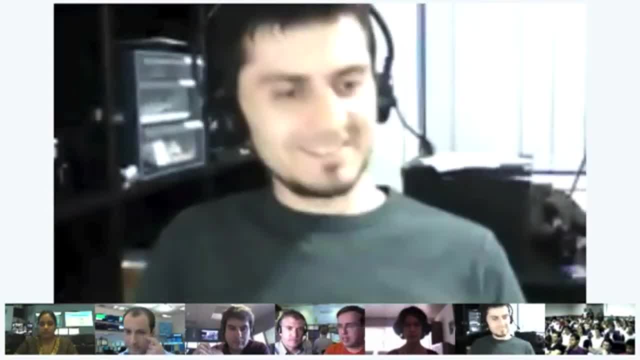 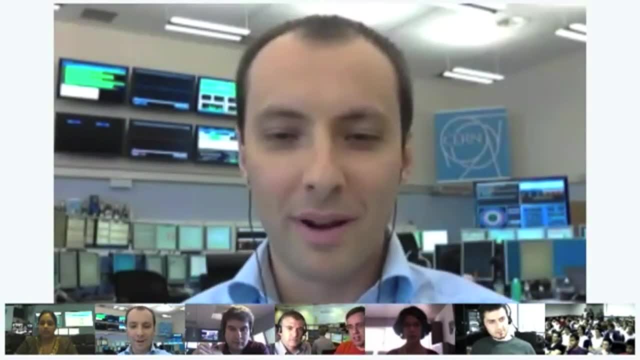 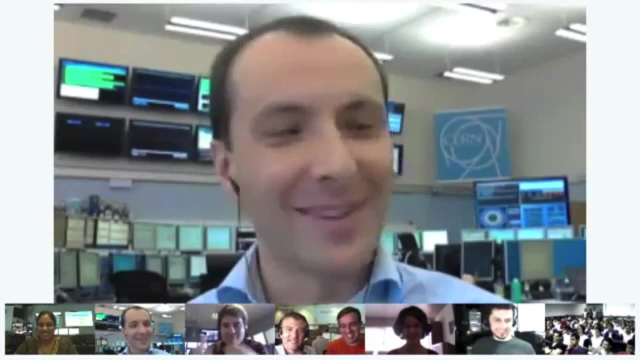 Right. so the technological bottleneck? Sorry, go ahead. If I may add something, Yeah, because I have the impression from what they say that we provide you crap, collisions with the product, which is not the case. We provide very good, very good, very, very energetic. 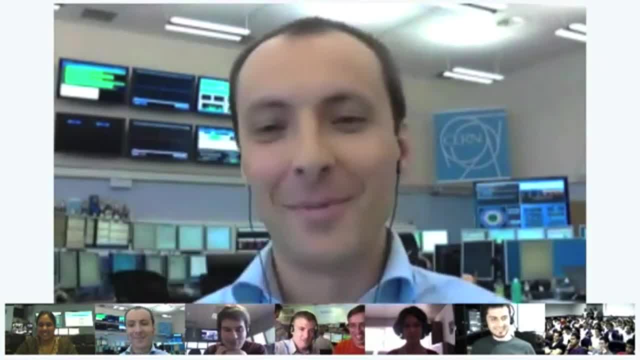 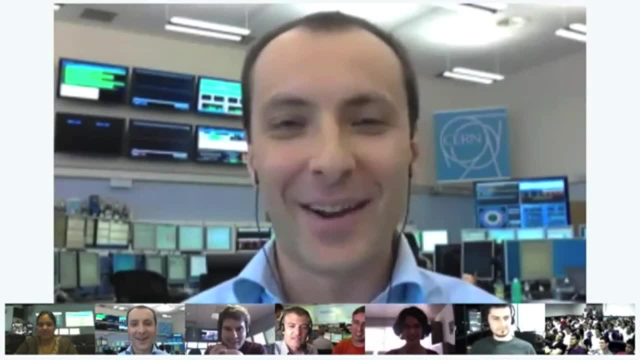 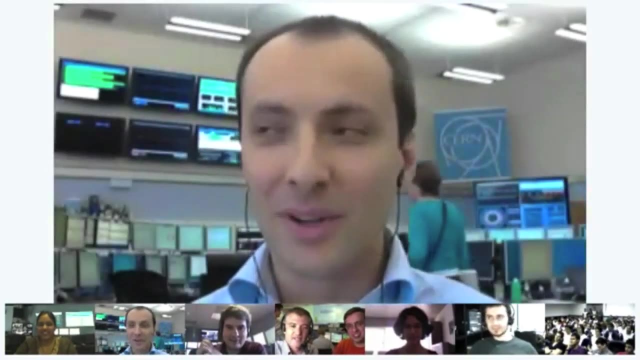 very dense beef. Yeah, that would be nice, Perfect, Otherwise, I would say we could work only a few minutes a day instead of being around the clock all the days for 10 months. So we have very good quality beams, but of course, your. 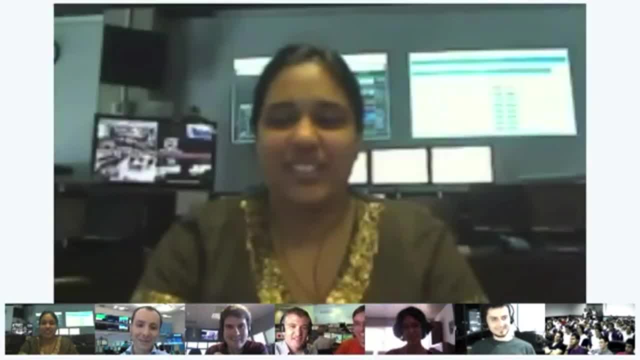 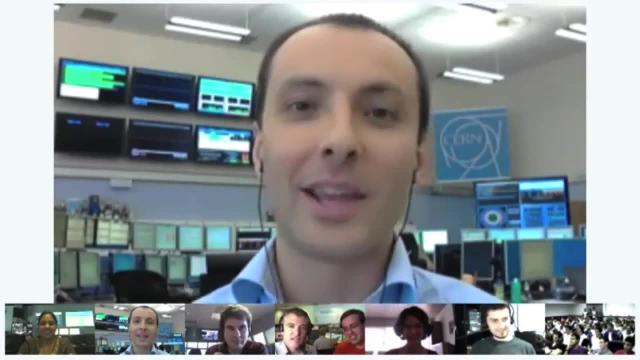 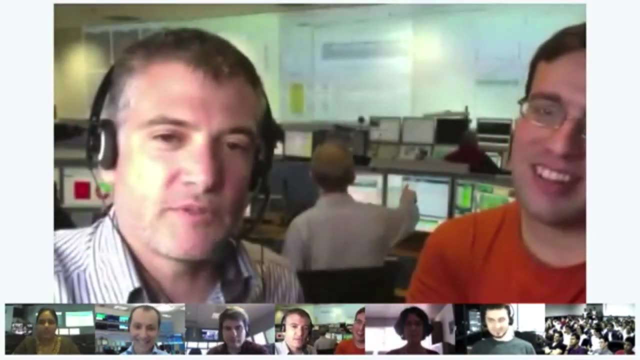 choice is to. I would say it's essentially your choice to decide and keep only a very small percentage of the collisions, making only the extremely good collisions that we'll have in the machine. Yeah, maybe, if I can add, do we have enough? 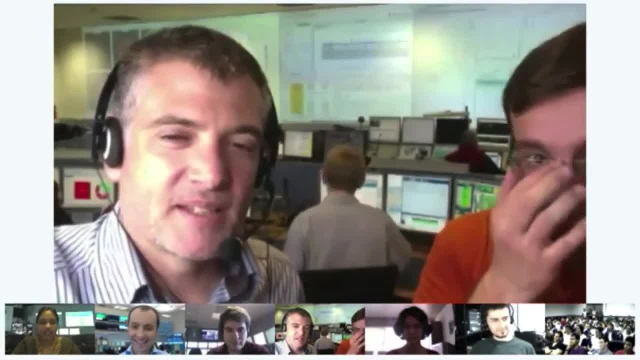 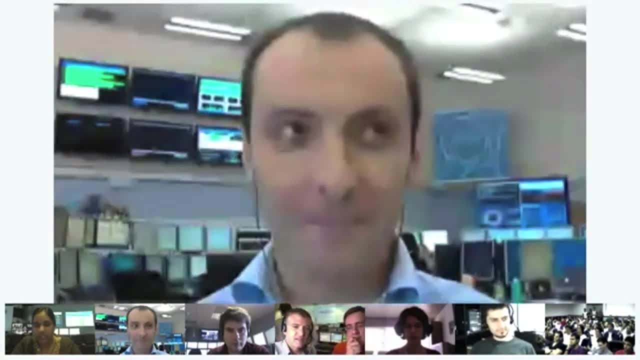 time to add a comment. Sure, yeah, We're going to extend this Hangout till the end of the day. I think we have about 60,, 40, but I do have a question for Mirko before we leave. so I think we have two minutes more. 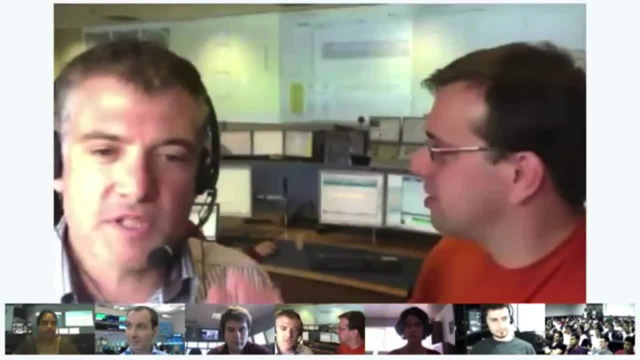 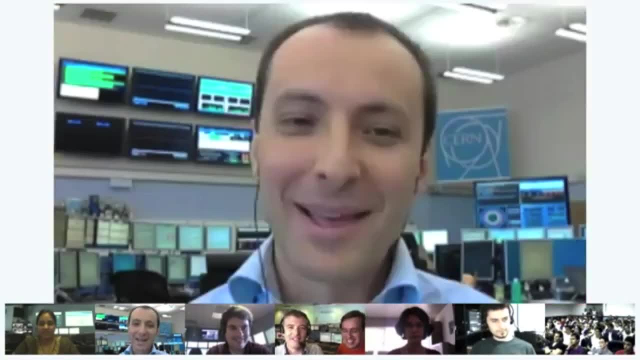 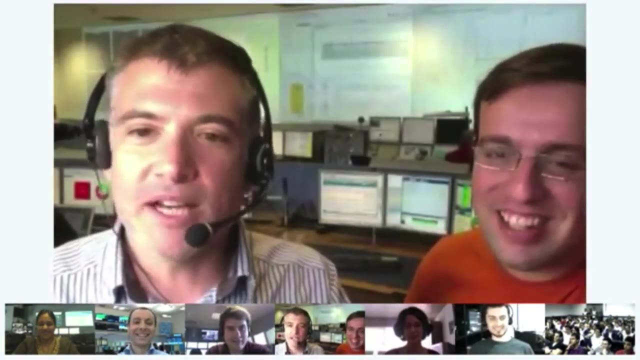 for comments: yes, Okay, so let me just add this comment, just to make sure it's clear about what we throw out when we keep The vast majority of these wonderful, incredible collisions that we get from the LAG, regardless of how well they are, a lot. 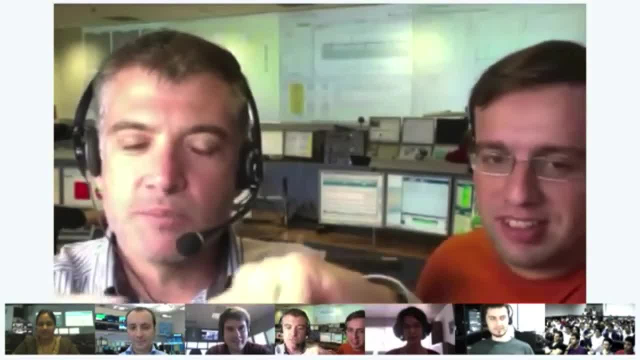 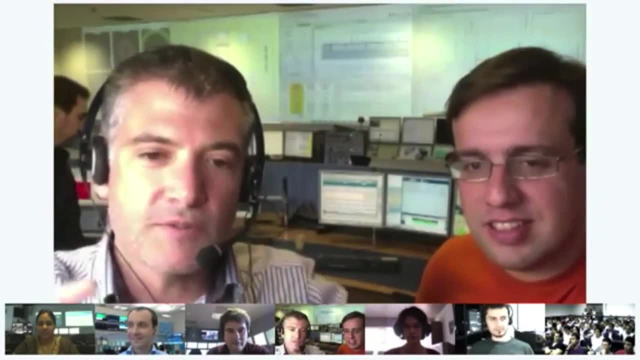 of the times when the protons come together, there's just a little scattering. that happens, and that's the kind of physics that we've already studied before. so the vast majority of the stuff that we're throwing out are things that we already understand. 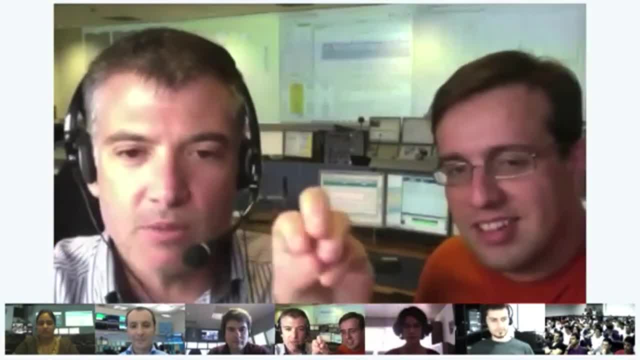 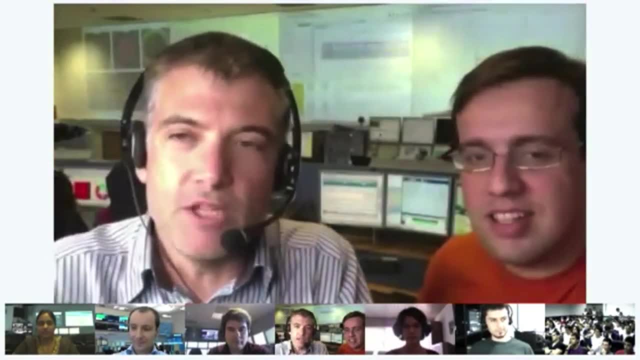 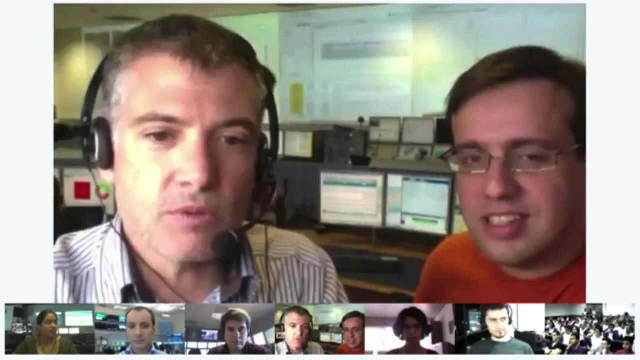 It's not that we're just really being very picky about what we keep. We have some what we call in our trigger of our selections. we call it a trigger menu. We have different items that we want to keep. We include in there some which are pretty general. 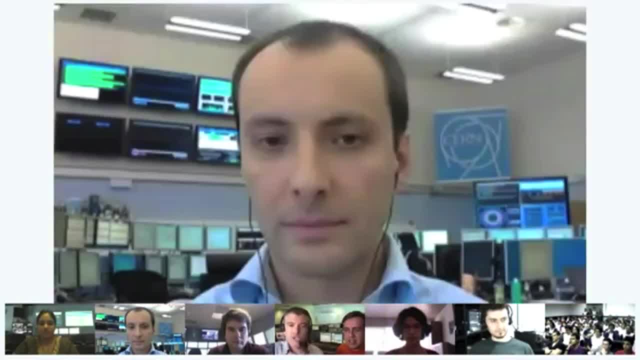 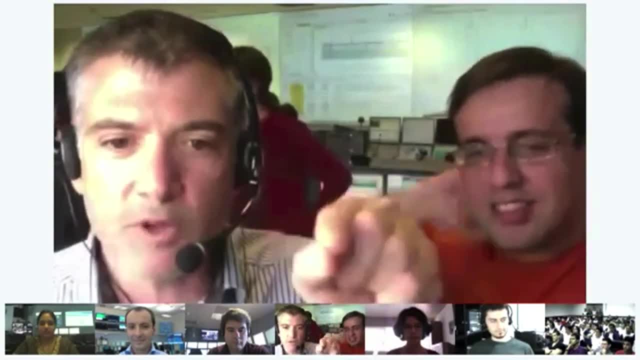 They just say we want to see what happens. Okay, We see that there are some hard jets coming out. you know that there's been a strong interaction and so we aren't necessarily specifically only looking for Higgs or Susie or these things. 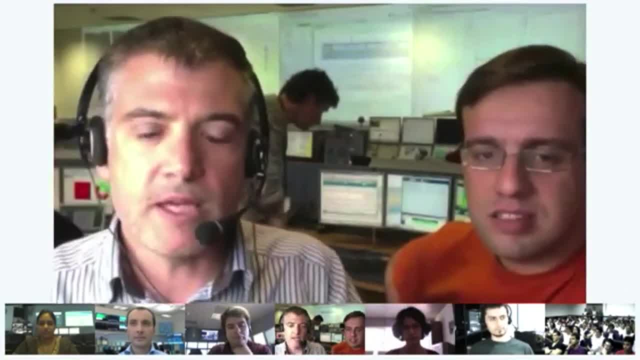 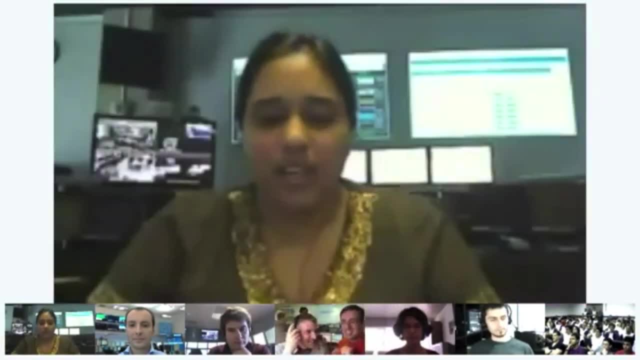 We also keep channels open for anything that's new, and we have a good idea from the past what that can look like. Yeah, and also, I think, just to finish this discussion, there's also an issue about what we do with the protons. 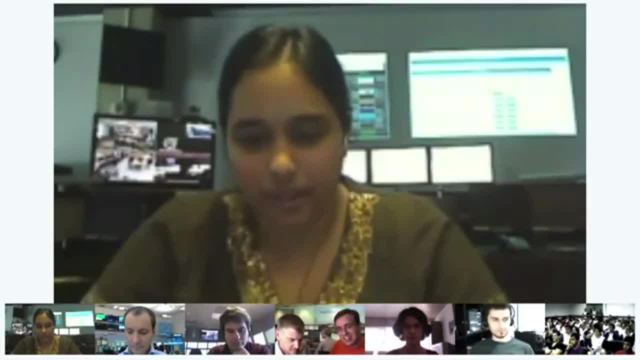 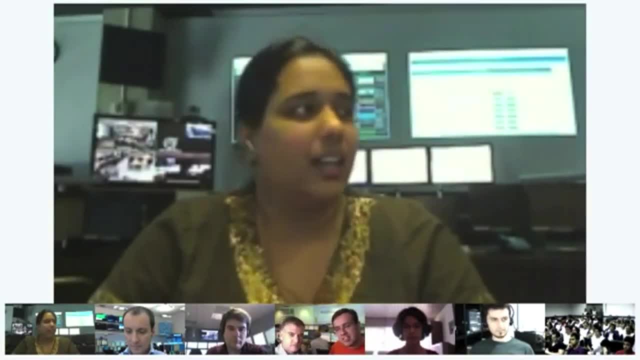 What we do with this data once we have recorded it and analyzed it for the first round, and that actually is a much more complicated question, and I think this is something both the experiments are still trying to decide on: what to do with the data in the very long run. 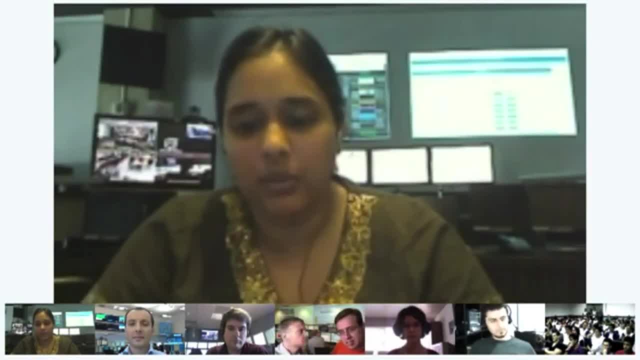 Of course it will be kept, and of course it will be kept in a way that it can be used or looked at again, but exactly what would be done with it is still being discussed, I guess I mean, if I'm wrong, David or Steve can answer that. 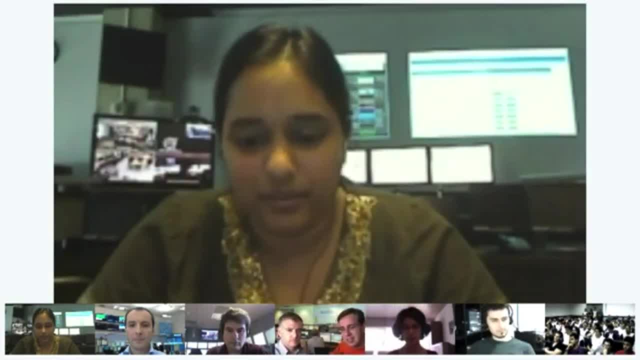 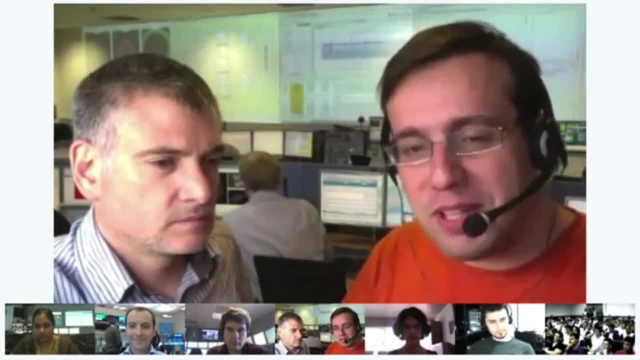 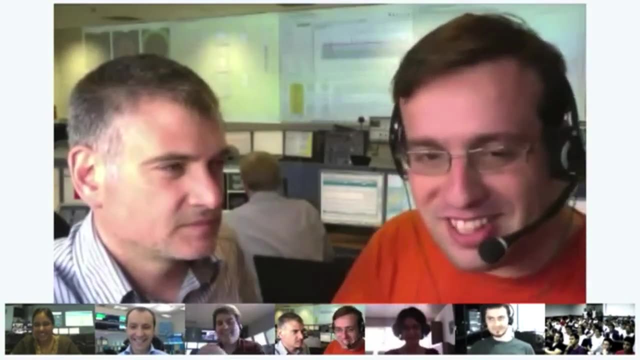 Okay, Okay, Just one sentence, a quick sentence. Our LHC colleagues, they really produce a wonderful beam, wonderful collisions. It's not their fault that we don't have all the collisions that are interesting. It's nature's fault at the end that for all the collisions produce a new Higgs boson. 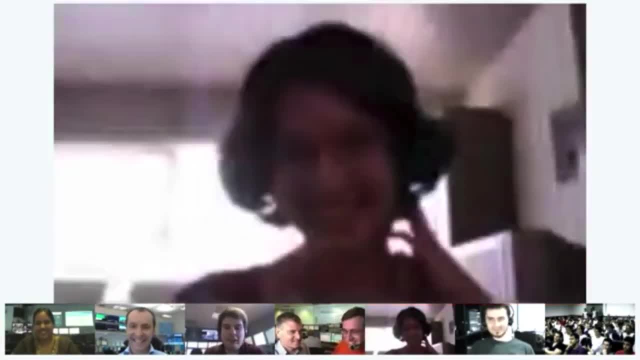 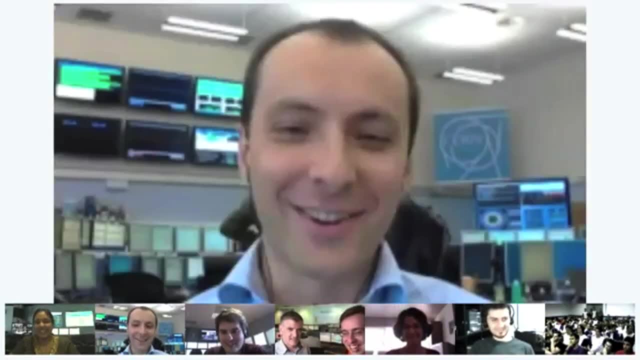 for example, and then we could go home in five minutes. Yeah, actually, what he's saying there is he's trying to make it so that Merco provides better collisions to Atlas than to CMS. I agree, I got that, Don't worry. 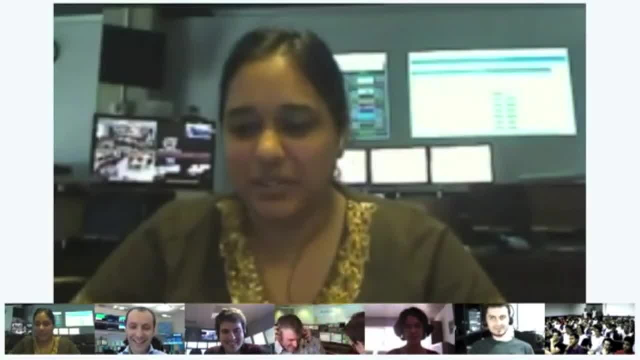 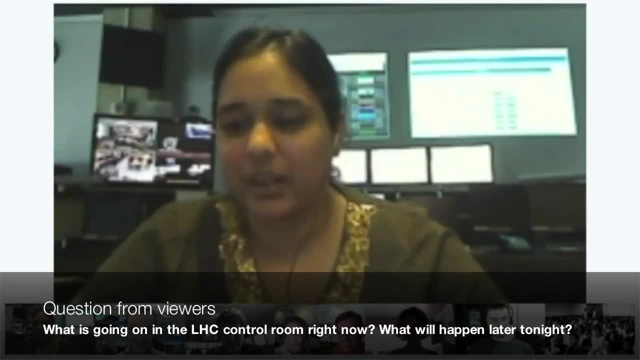 Got that. So now I have a question for Merco about now that we have the expert here. so what is going on at LHC control room right now? What will happen later tonight? Yeah, Maybe a little insight would be great. 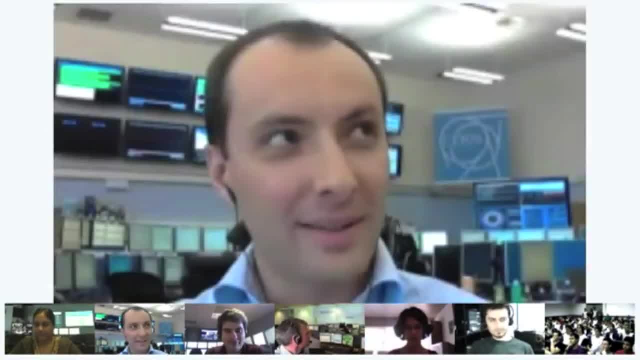 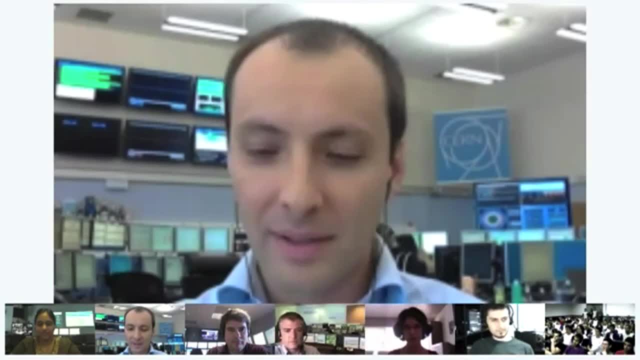 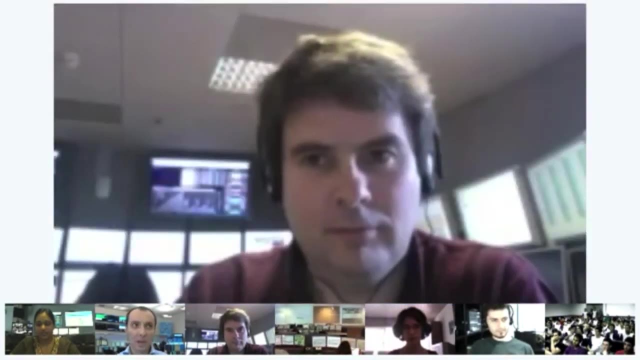 Yeah, Yeah, Yeah, sure. Well, the aim of today was getting the first table beams collision that is essentially going up with two, with three bands, Okay, Okay, Okay, Okay, Okay. So with three bunches on each beam, three packets of particles on each beam, up to 40. 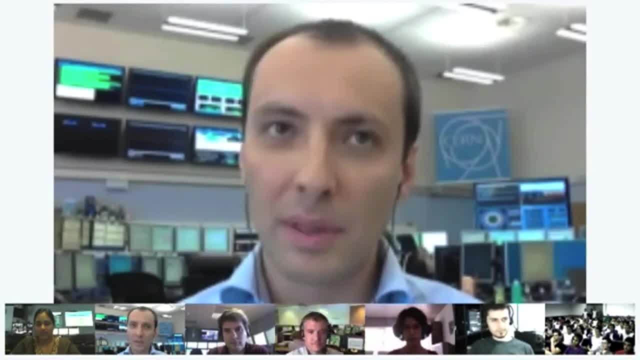 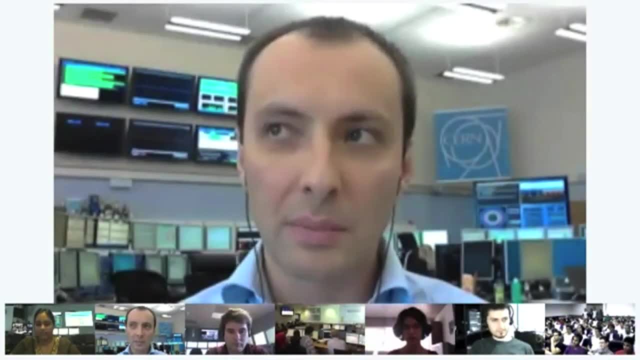 d, squeezing them down in the experiments and then making having them collide in the experiments and declaring what we call stable beams, which is a phase where we don't touch the beams and the experiments can switch on all the components and detecting, let's say, 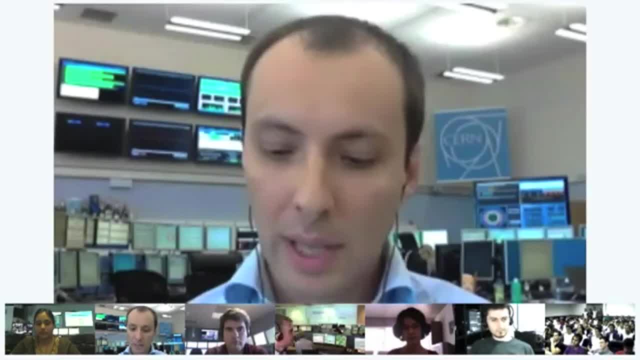 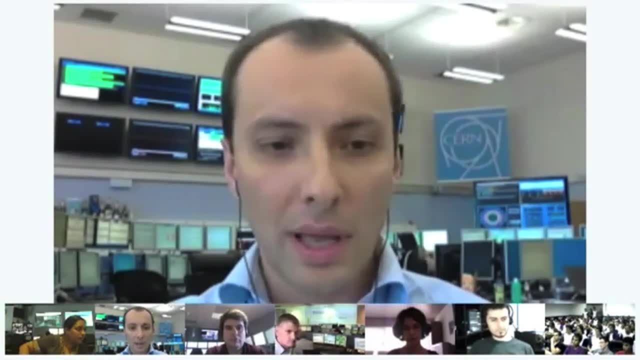 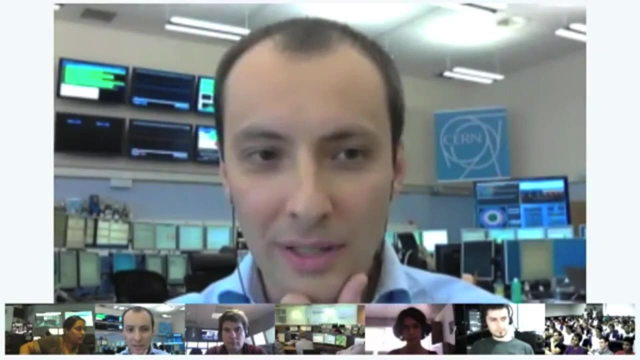 measuring all the events from collision. Unfortunately, we've committed some delays, Okay, Okay, So we've committed some delays due to some problem in the machine and also, if I Dave, just continuing on the history of faults on the detectors, I read in page one that we 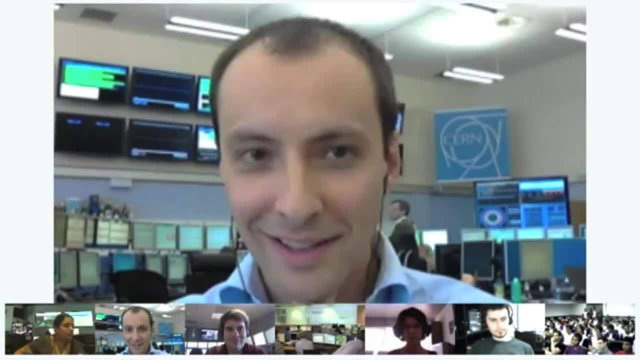 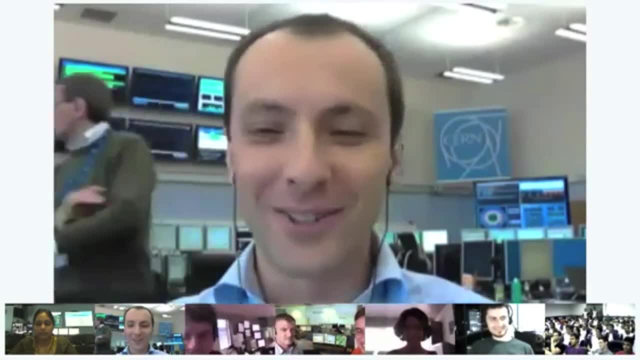 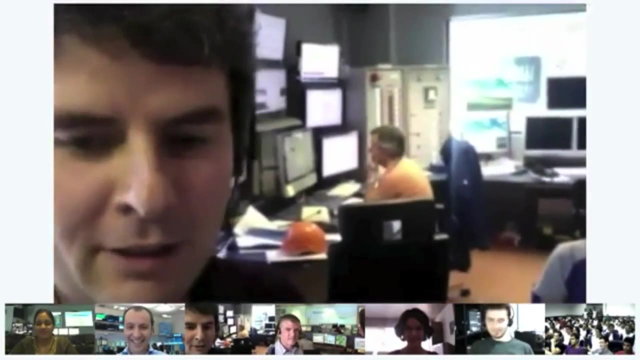 have problems with the CMS, BCM at the moment, And you can feel that, Yes, Actually also, not only the machine, but also the experiment broke down. Yeah, So in fact, my colleague behind me is Is currently working on exactly that.